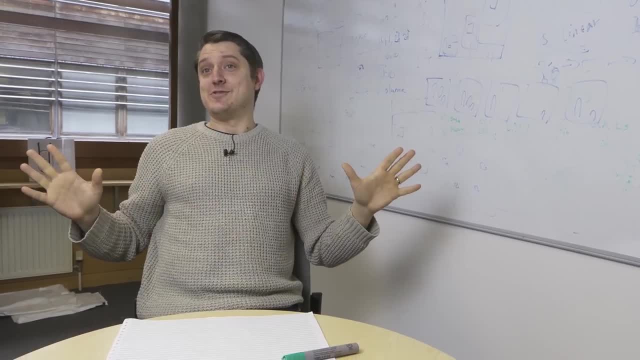 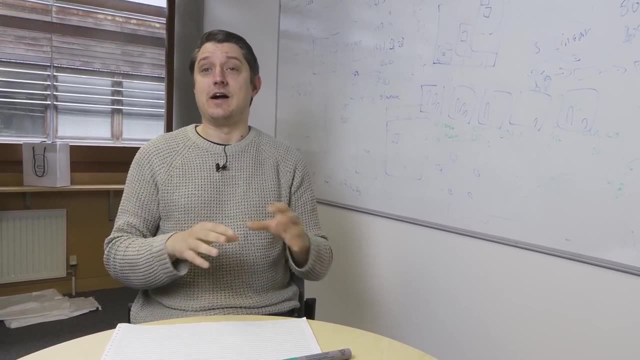 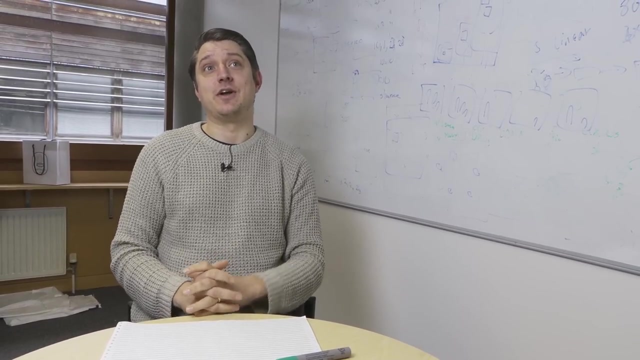 I thought, just for a bit of a change of pace, we could look at one of the classic algorithms: Binary Search. Binary Search is something you learn about perhaps slightly earlier in your career, maybe as an undergraduate or maybe even in school, But it's super important and, I think, also really interesting because it illustrates some of the things you need to think about as a software developer. 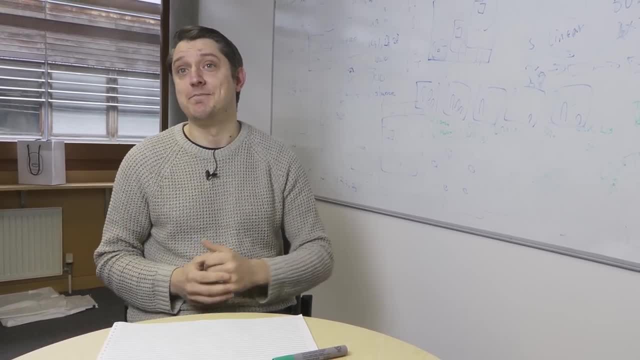 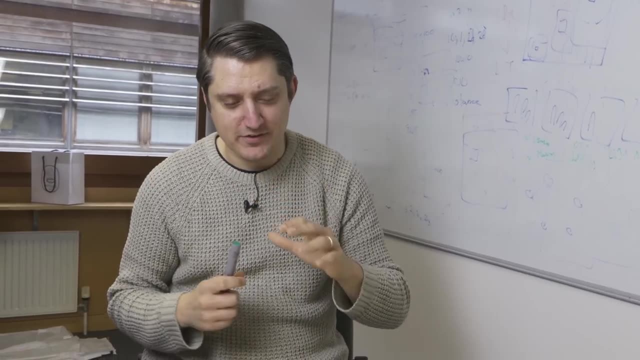 about how to make things faster and how to use things appropriately. So that's what we're going to look at today. All right, So let's imagine we have some boxes right? So it's like deal or no deal, sort of like that. 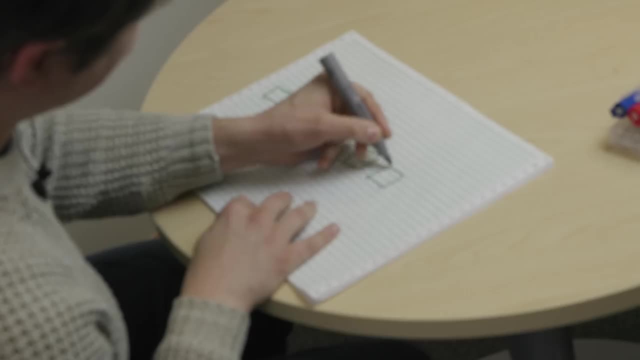 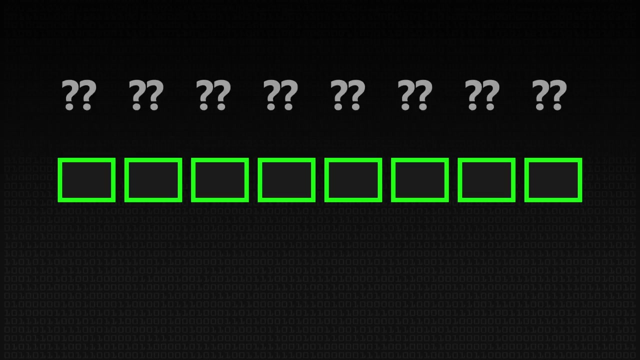 But that analogy is going to break down pretty quickly. So I'm going to draw some boxes. I could have pre-drawn these, but where would be the fun in that? Now you don't know what numbers are in these boxes. It could be any number on Earth, Any number on Earth. Is that a thing? Any number? 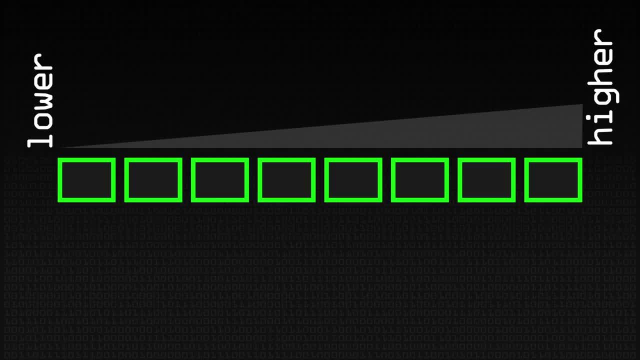 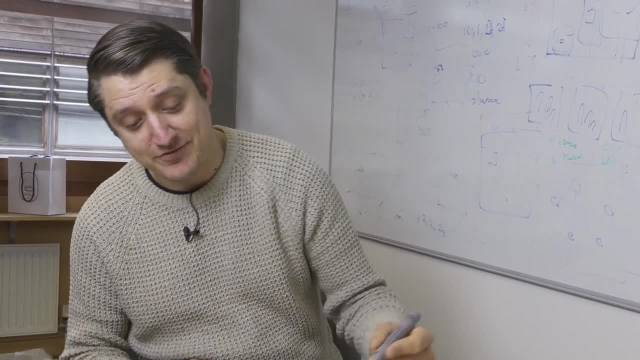 But we do know they're in order. So the lowest number is here and the highest number is over here. Let's say they're introduced just for the sake of me not giving myself a headache. Now. I want you to find out if the number 17 is in one of these boxes. 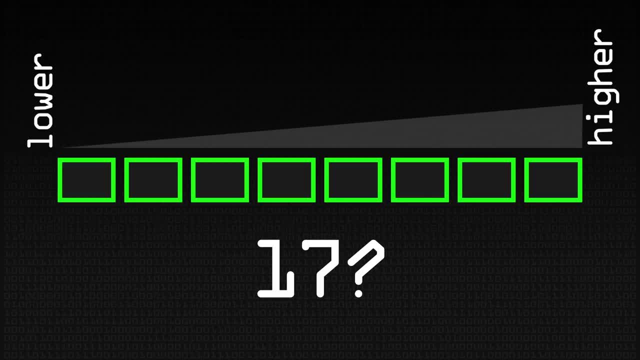 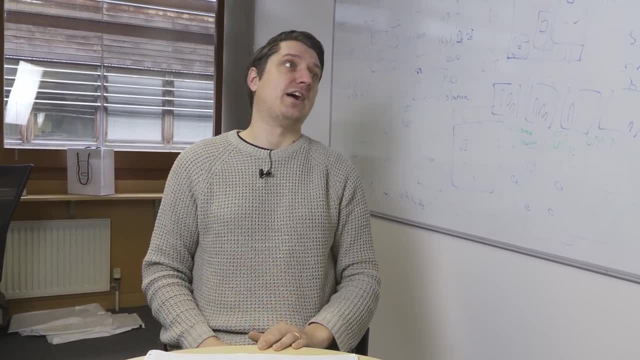 That's the thing you need to do. This is what binary search is for, but just searching in general. So maybe you've got a database with a bunch of IDs and you need to look up a specific person's ID or you need to find out anyone who's born on a certain date. 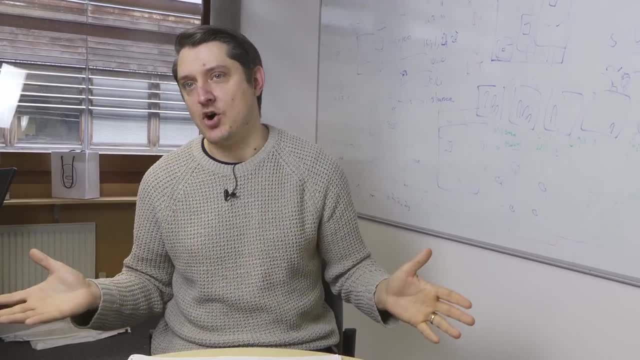 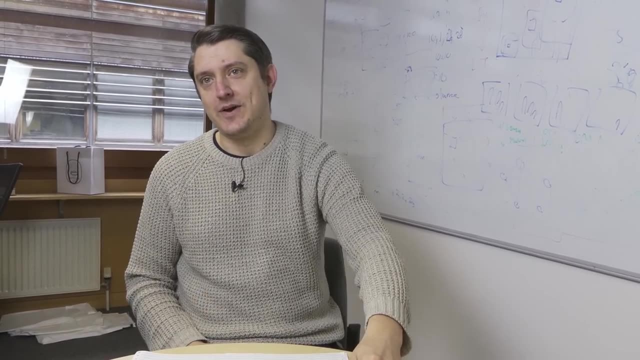 Looking through data to find something is very, very common. This is just one way of doing it. So that's the rules, right. The boxes are ordered. How do we find this as quickly as possible? The naive approach will be: we start on the left right. Let's just open this box. 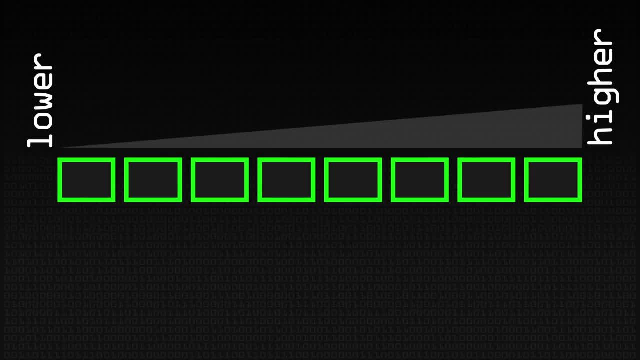 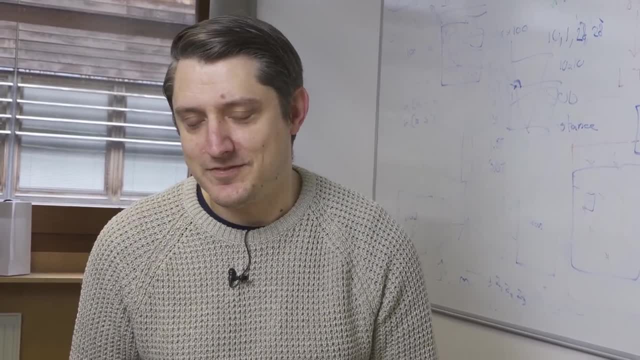 Let's not do anything clever: Open the first box. The first box is two, So it's not 17,. so we've failed badly, but we are at least slightly closer to the goal, because now we only have this many boxes to open. 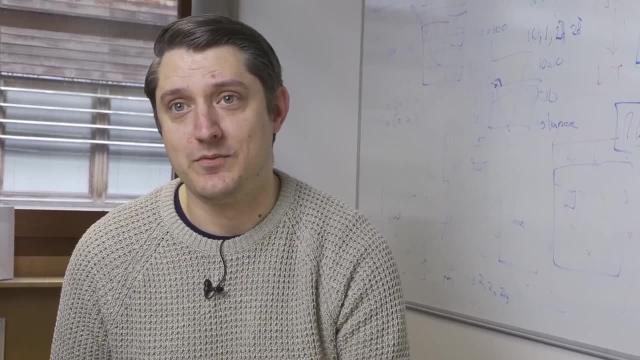 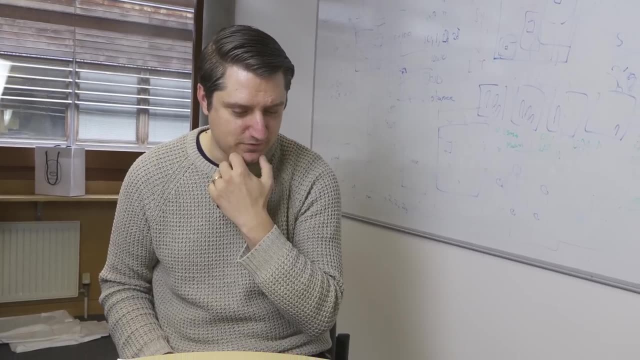 So let's think about that. How much easier have we made this problem? Well, it was, what was it? eight boxes, Yeah, seven boxes. now We've made it one box easier. It's not trivial. So the best case from now is 17 is here, We open the box 17,. job done. 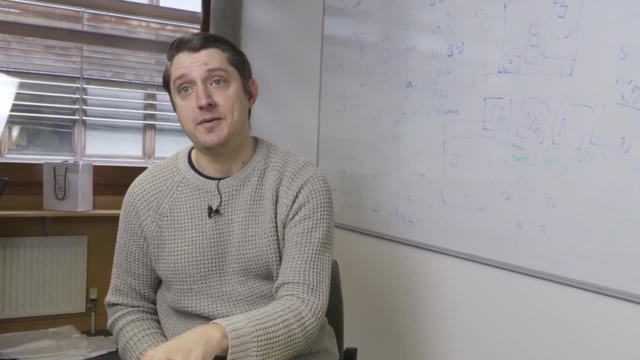 The worst case is we look through all of these boxes, one at a time, And 17 isn't in there, right? Or it's right at the end, or something like this. I'd think I'd divide and conquer, I'd go somewhere in the middle. 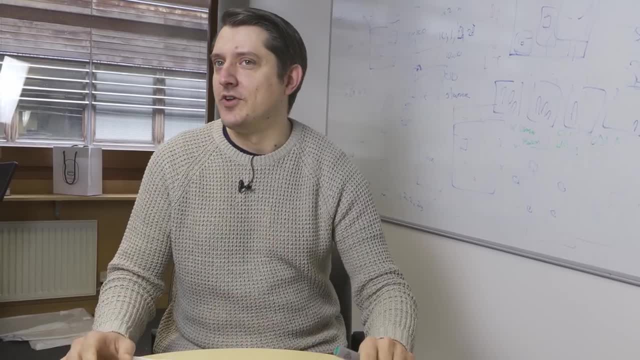 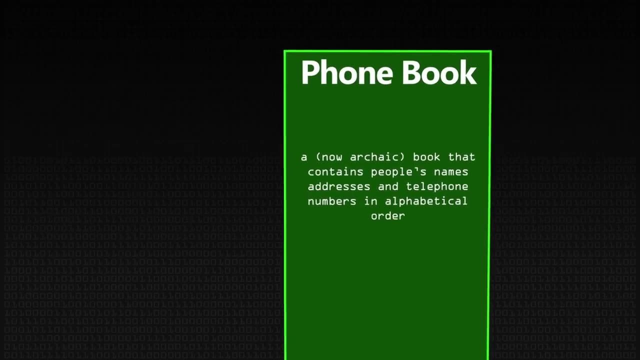 Yeah, I think you should divide and conquer, right? So if we know they're in order, we can start looking at it, a bit like you would look through a phone book, right? You'd open a phone book- You don't open a phone book- on the first page and start: come on. 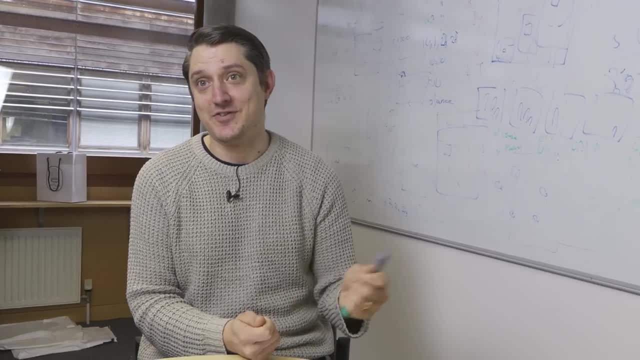 I mean, I know their surname begins with Z, but I've started so I'm going to finish this right. So let's open up a box around here, right in the middle. I've chosen an even number of boxes. 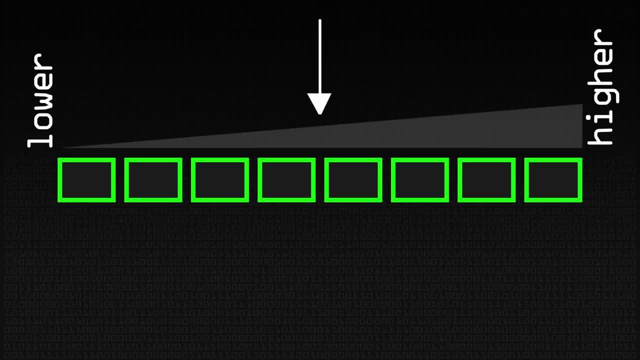 So let's just sort of Do this one right And okay. so we open this up and it's not 17.. Let's say it's 16, which is awkward, but sure, Okay. so now, what have we learned? How much easier have we made this problem? 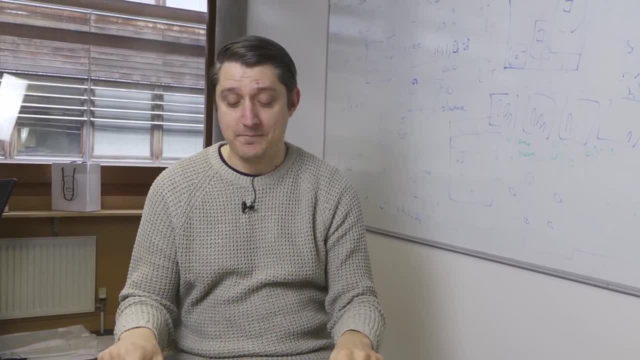 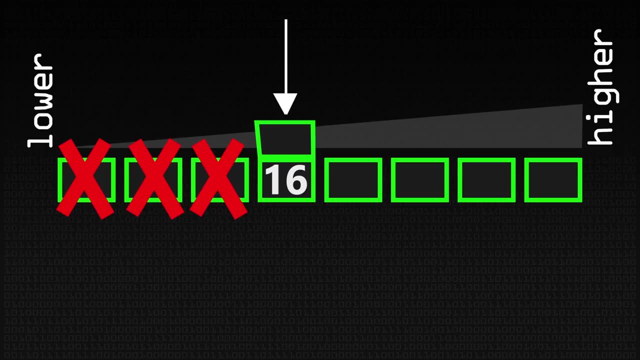 Well, we know now that, given this is in order, that 17 cannot appear here and here. right, Let's presume we haven't opened two. It can't appear here. either It has to be in one of these or not in the set of boxes at all. 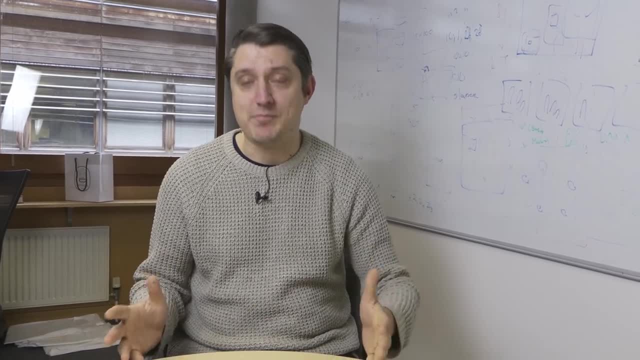 So how much easier is our problem? You've halved it, right? I've halved our problem, yeah, but our problem is double as easy, You know in some sense. So now let's fall back to our rubbish algorithm. 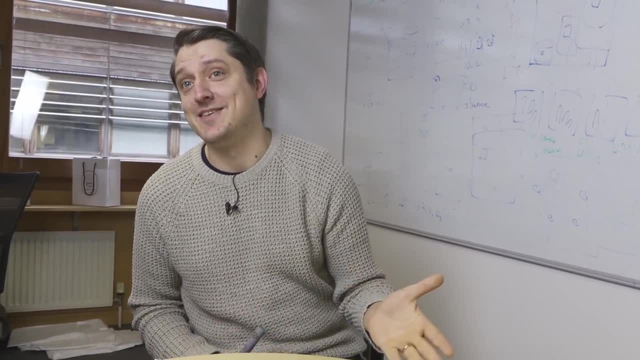 We'll just open this one and then this one, and then this one and this one, Or we can repeat this process. That would be much better. With 17,, you would assume it is going to be the next one, unless there's another 16.. 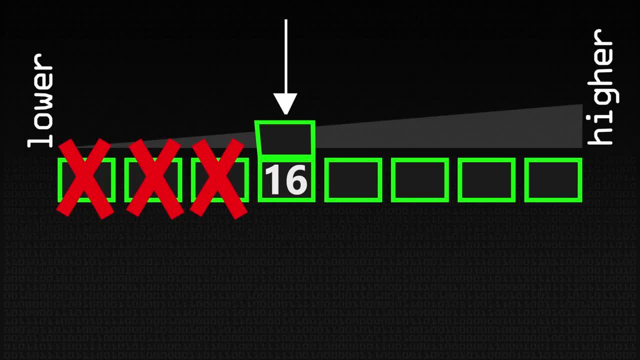 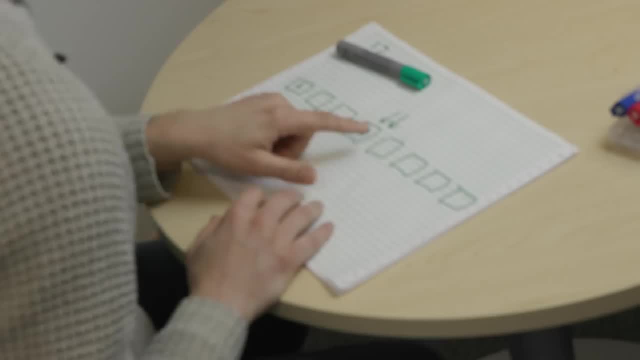 That's true. Actually, 16 is a terrible, terrible example. for that reason, Let's make that 10, right, Fixed, fixed, Delete all that bit of video. right, This is 10, so we don't know now, no, 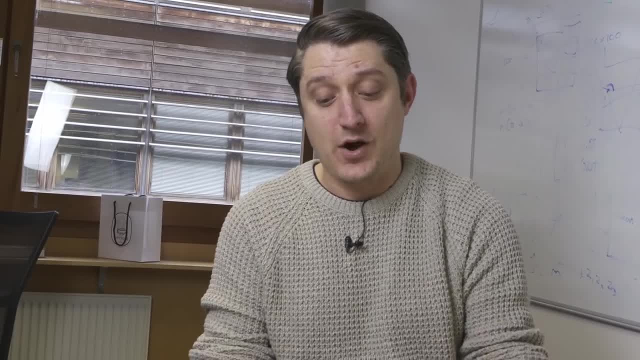 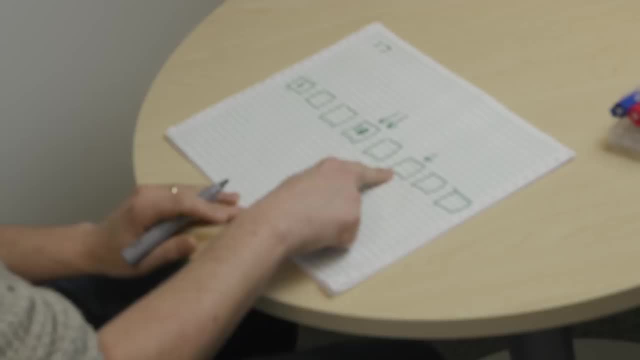 The point is we're trying to make a general algorithm, right? We don't know what this number is. All we know is 17 was bigger than it. So now we're in this half. yeah, So we jump halfway. so let's say this one, right? 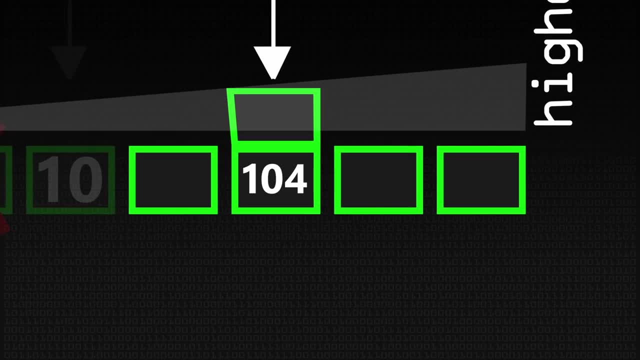 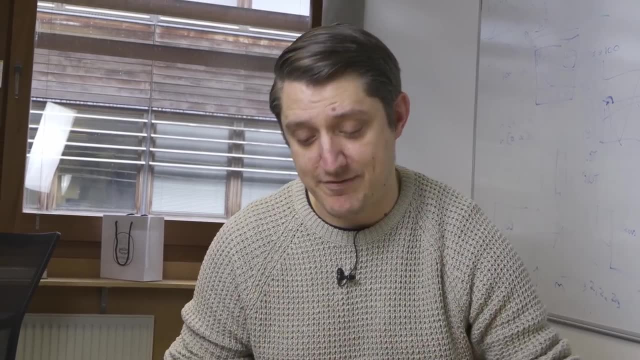 And we say, okay, is this bigger or smaller than 17?? Well, it's 104.. So we now need to go to this half right, And we're halving every time. We're halving our problem every time. 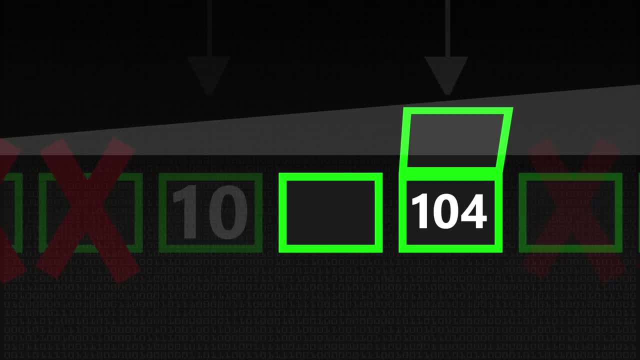 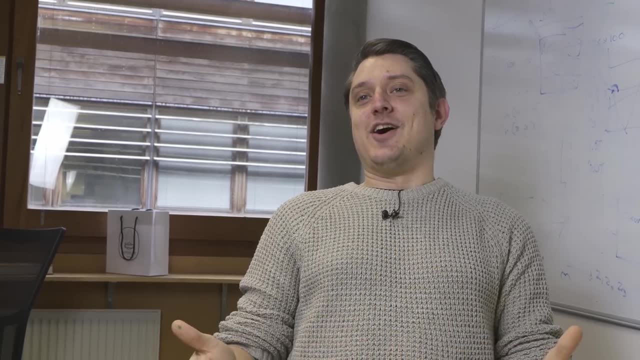 And we look in here, Is it 17?? And you know, let's say it's 16.. Oh, 16 has come back And so, no, 17 isn't in this set of boxes. Now you know, you might be thinking I should have done this ahead of time. and then you know, come up with my example better. 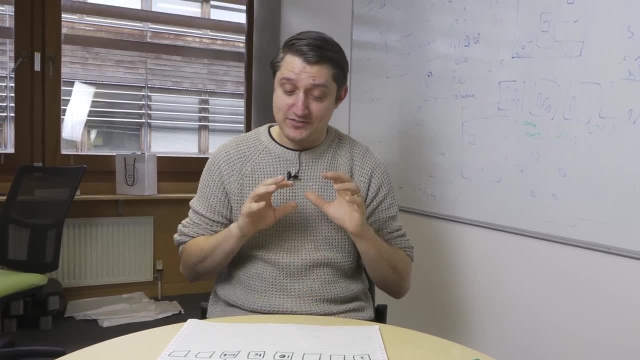 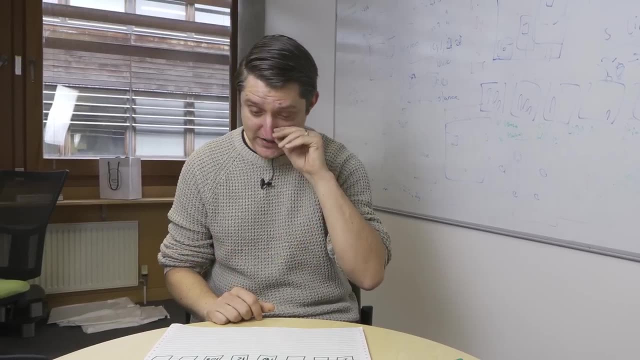 But the point is that we can make this much, much easier by dividing and conquering right. If we know these are in order, which, to be fair, is a big ask. sometimes, depending on the data, we can zero in on our target number as quickly as possible. 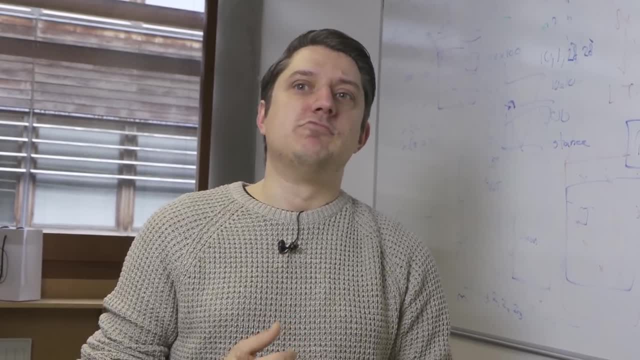 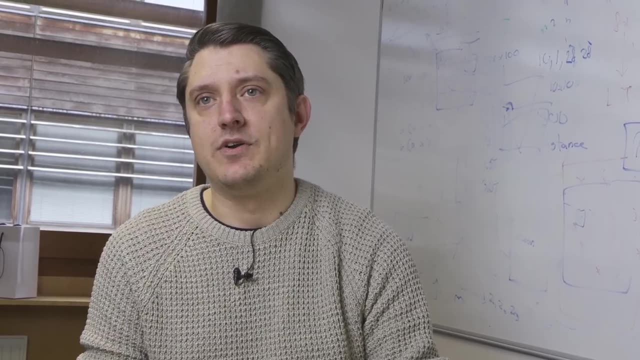 So how much easier is this. Well, what was the running time for the linear search, which is just going like this right? Well, it's going to take exactly how long the number of boxes is right, Or, you know, we might get lucky halfway. 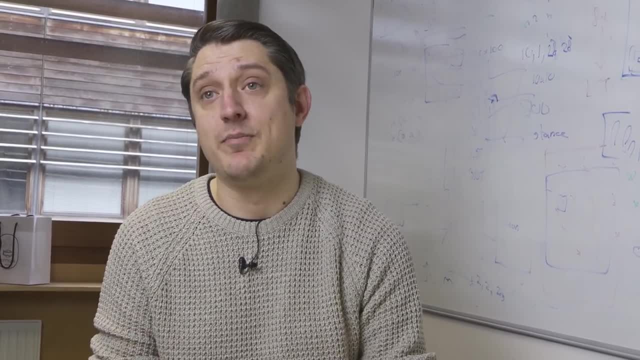 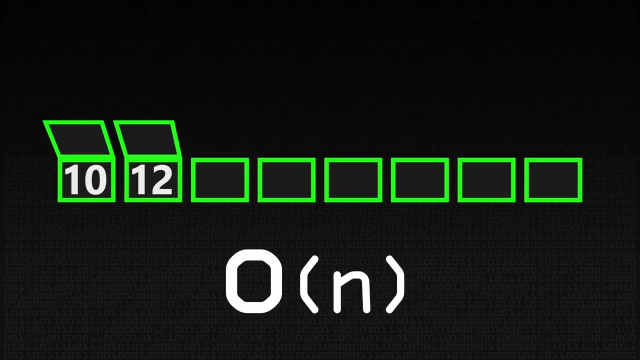 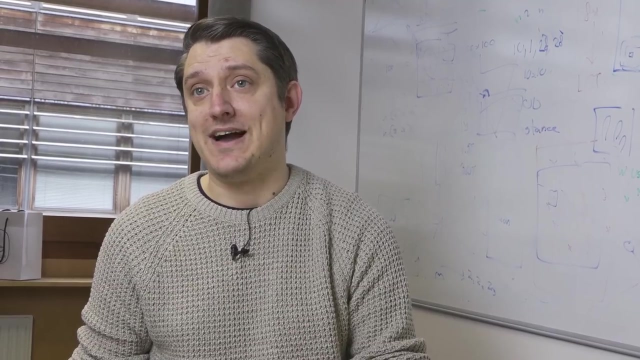 We might not, But you know, in the worst case it's going to need all of the boxes to be searched And we're not going to find the number we're after. So we call that O of N, right? So that's saying, but roughly speaking, the amount of time a linear search will take is directly related to how many items we have. 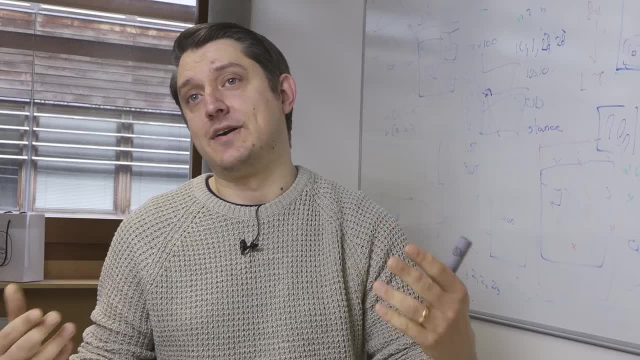 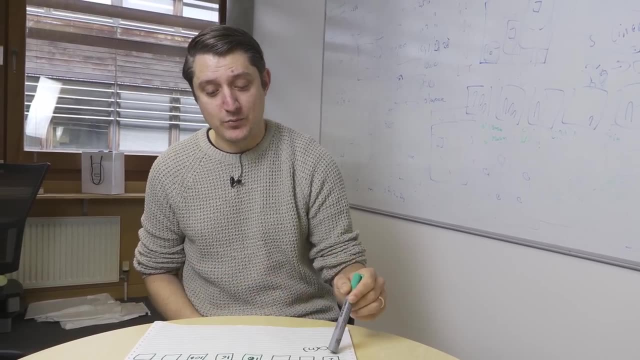 Now this is not very many items, But if you've got gigabytes worth of data, that's a lot of searching to do. So how much easier is this When we're doing binary search? So we're dividing by two, and we're dividing by two again, and then we're dividing by two again. 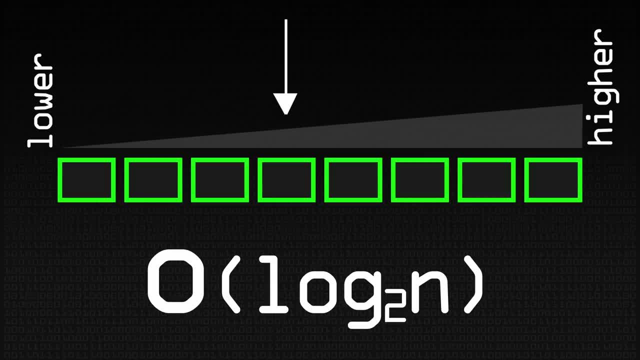 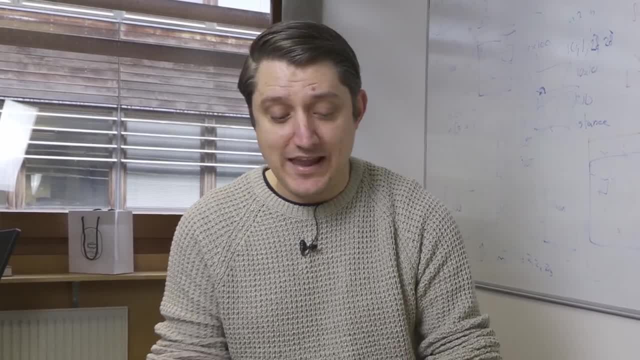 Well, actually it's O log to base two of N, And what that's basically saying is that as N increases, our problem doesn't increase at the same rate, Right? If N doubles, our problem only gets one harder. So suppose we have a billion numbers, right? 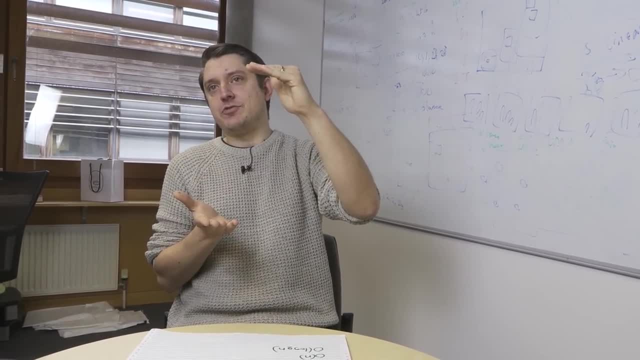 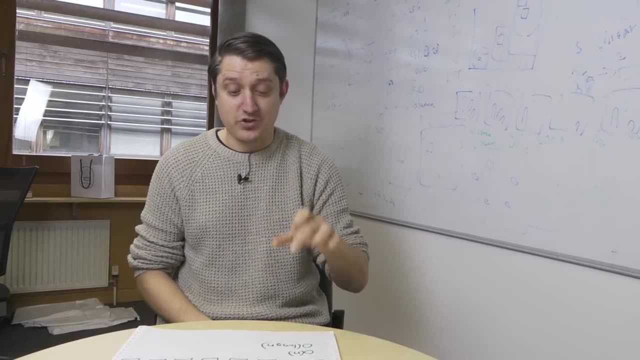 And it's this hard. If we have two billion numbers, we just have one extra step because we have to do that first divide to get down to a billion numbers, Right? So it's so much more efficient and it scales so much better. 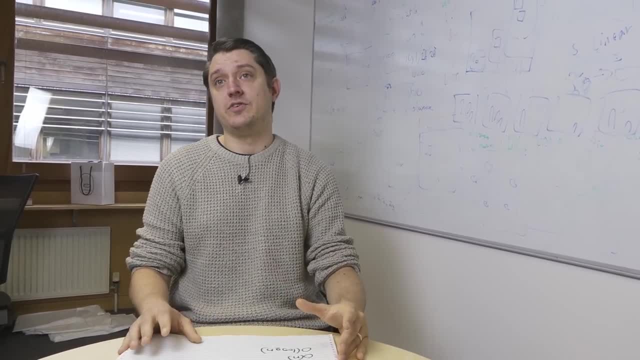 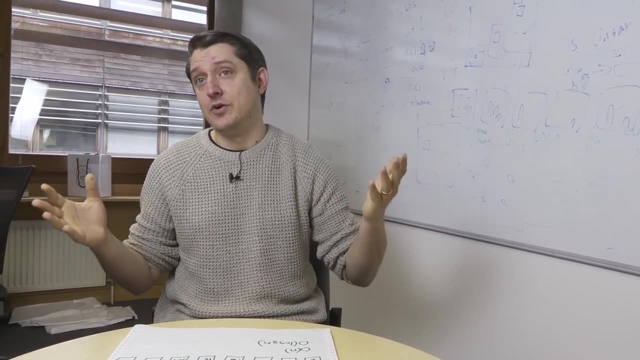 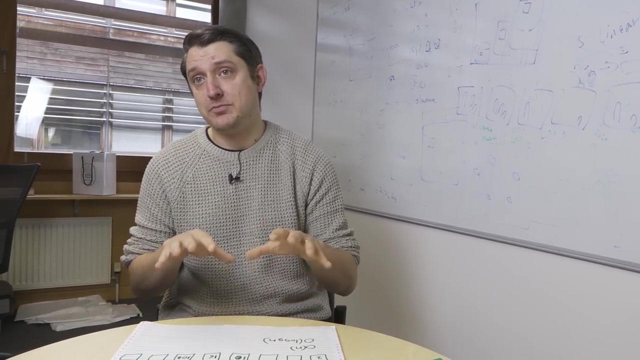 Scaling, really, I think in these kind of algorithms is what's important. It doesn't matter how long this takes for two numbers, right, Because you just look at them, It's not a huge deal. But when you've got billions or you know even more of numbers that you've got to look through, being able to do an algorithm like this is going to be much, much better. 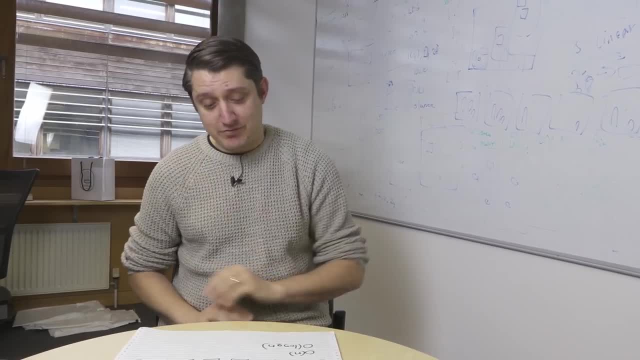 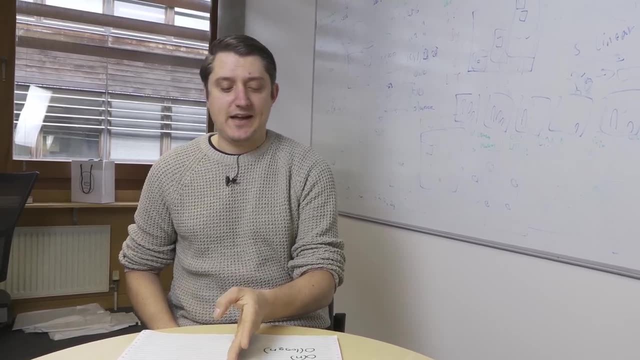 Right. So how would we program something like this? Well, what we need to know is we need to be able to basically be able to calculate the midpoint. We need to calculate the midpoint of where we are Right, And so the first time that's easy, because it's just the length of this array divided by two. 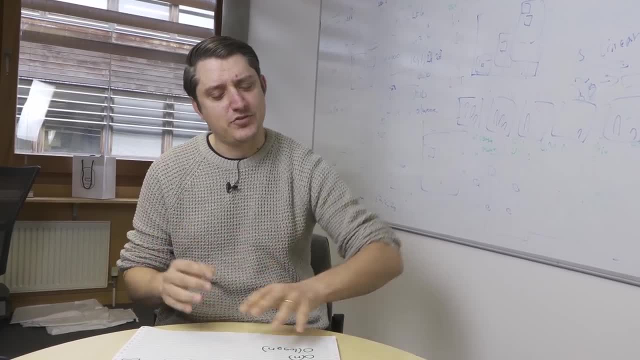 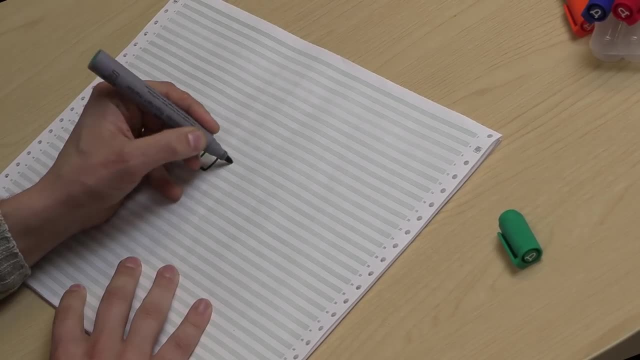 Right, But actually we want to be able to generalize this a little bit, So it would be helpful if we have a couple of variables that determine where we are. So let me draw out some more boxes and we'll do it fresh. Speed this bit up. 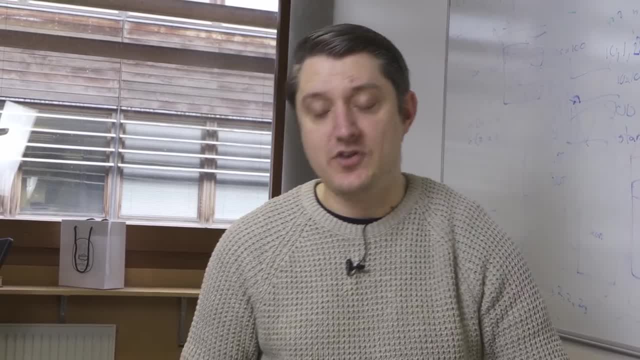 Okay, They got less good as they went through. Anyway, we need to think about how we're going to implement binary search. Right, We're looking for some number- Let's say it's X in this list- And we don't want to open the first one and then the second one. 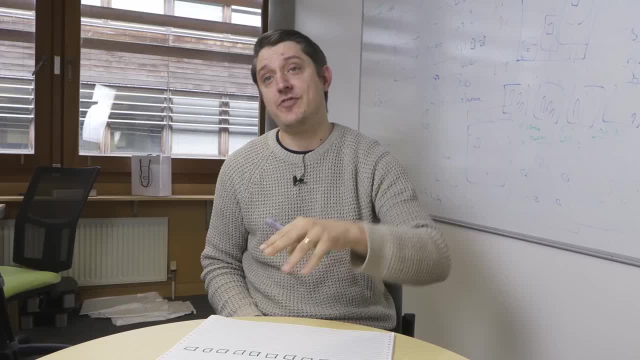 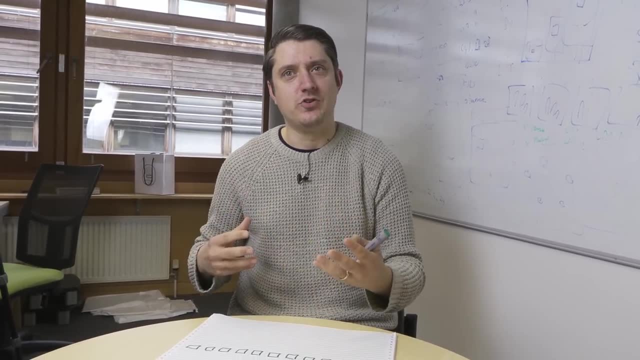 That's linear, That's binary search. We want to divide and conquer. We want to go halfway. Now the first iteration would be quite easy: We just take the length of this list divided by two. But actually we want a more general solution, depending on which bit of this problem we're solving and how many iterations we've run already. 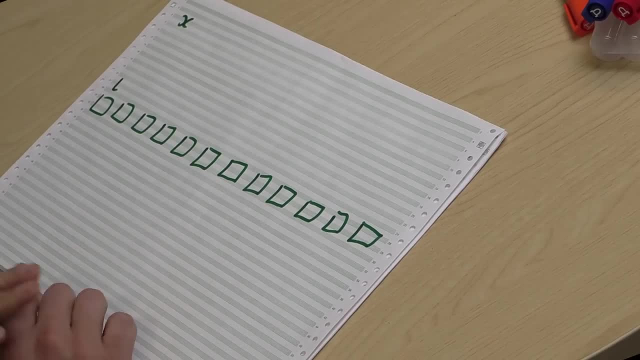 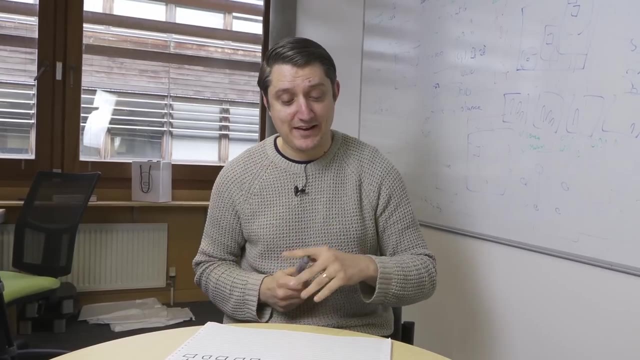 So let's define a couple of variables. Let's say the left is the leftmost box we're considering And the right is the rightmost box we're considering, And we initialize them as being the first element and the last element of our list or our array. 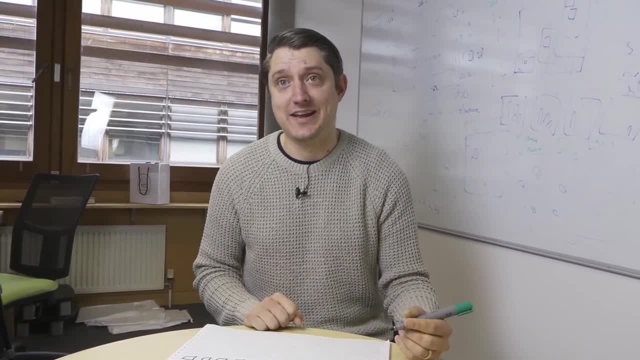 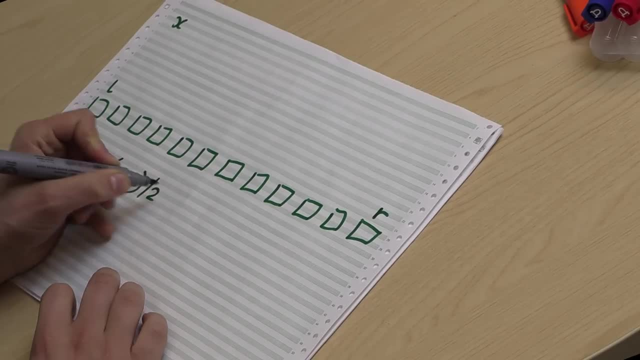 So then we can calculate the midpoint, The first one we're going to look in, as M is equal to L plus R divided by two, And then that might be depending on 1,, 2,, 3,, 4,, 5,, 6,, 7,, 8,, 9,, 10,, 11,, 12, 13.. 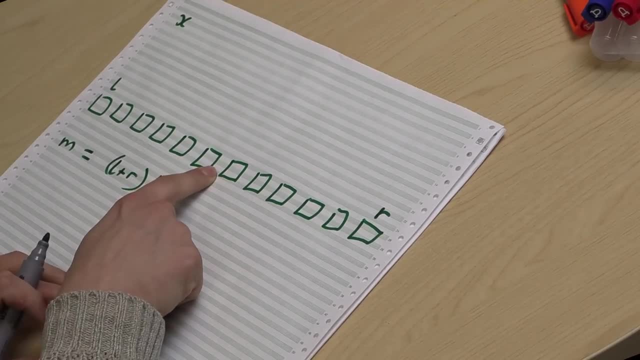 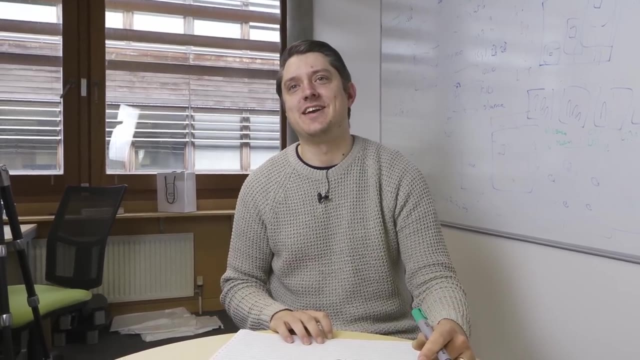 It's actually, I think it's this one. No, it's not, It's halfway between these two. If L plus R, does that mean L, as in the number one? One plus Yeah or zero, depending on whether your indexing is. 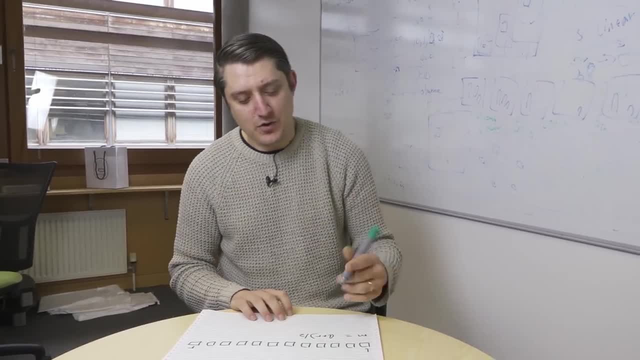 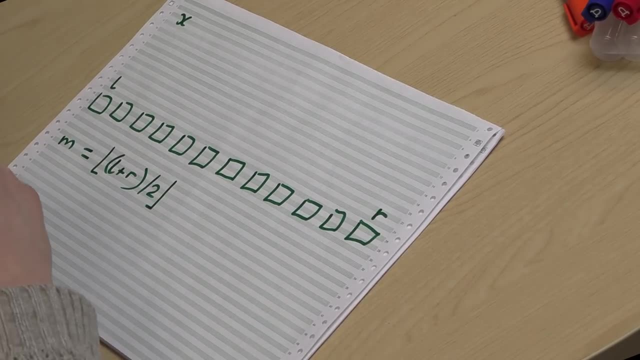 It depends. You know what I mean. Yeah, yeah, But we don't want to arrive halfway between two elements, So we'll just do the floor function here. So we'll round down to the nearest integer, We'll discard all the extra bits. 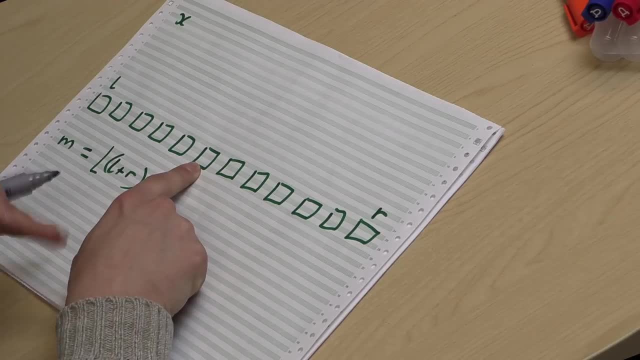 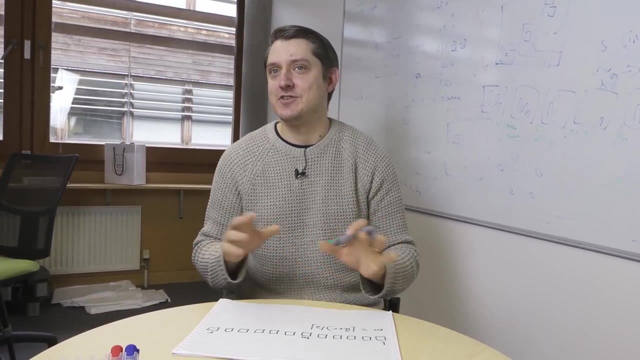 And so we're going to end up. I think here I'm not actually counting now, I'm just going to guess. So this is M. Now we open this box, or we look in the array, or we read the database entry, or whatever it is we're doing. 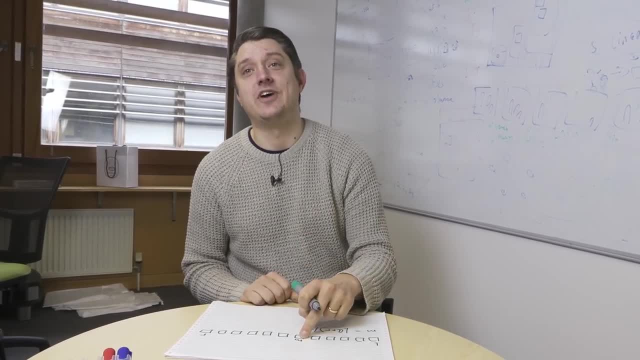 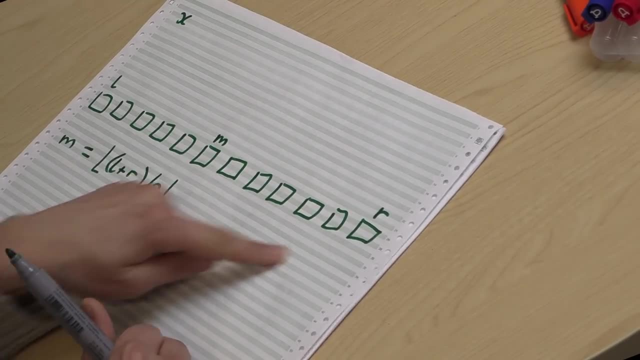 And we find out that X is not equal to M, So we haven't finished. And we find out that X is bigger, Which means that X must be in this region here, if it's in this list at all. We also now know that this is not this. 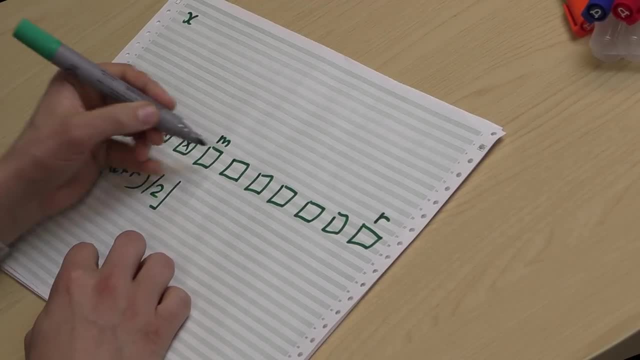 It's not these, It's not these And it's not this one. And we also know it's not this one because we just looked And we haven't had to look at any of those, So we've saved a huge amount of time. 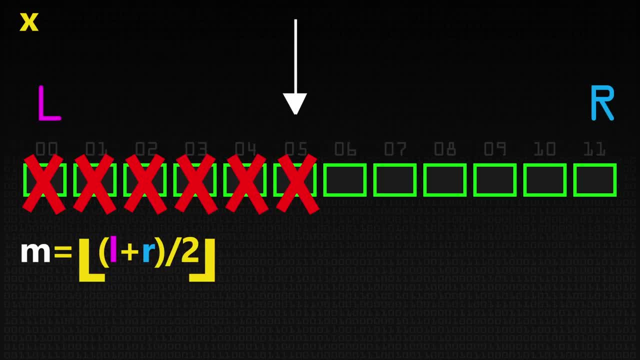 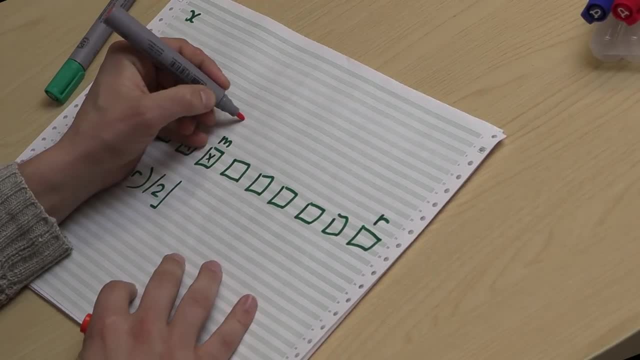 So the next iteration, what we need to do, is we need to move our left-hand side over to here, So that we're now looking in this region. So I'm going to change color Controversial And I'm going to say, okay, L is now. 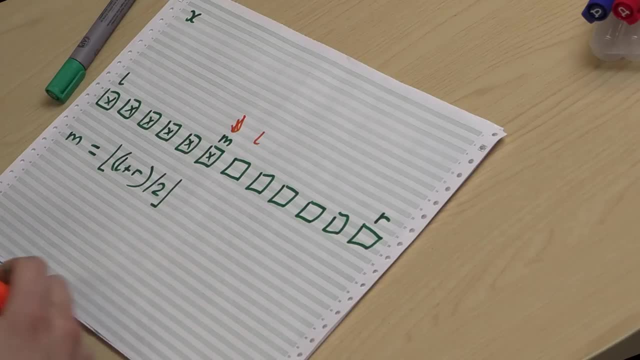 Not there, Excuse me, It's there There. No, We've already looked at that one. We don't need to do that. So then, R, it stays where it is All right, And then we create a new M. 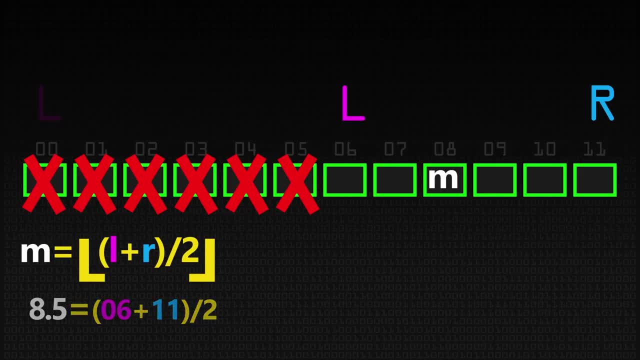 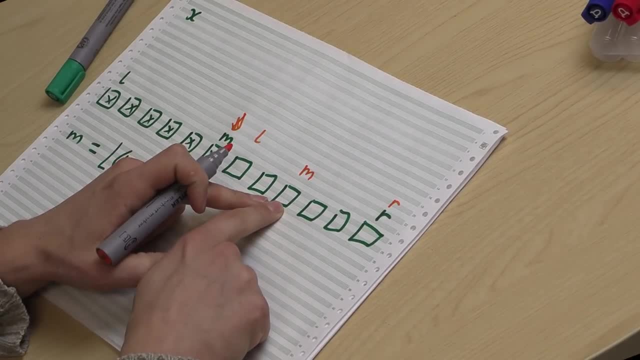 So we do: M is equal to L plus R divided by 2.. And that ends up here. So let's do our new M And we look in this one and we say, okay, X is actually smaller than this. So what we've done there is: we've discarded this one, this one, this one and this one. 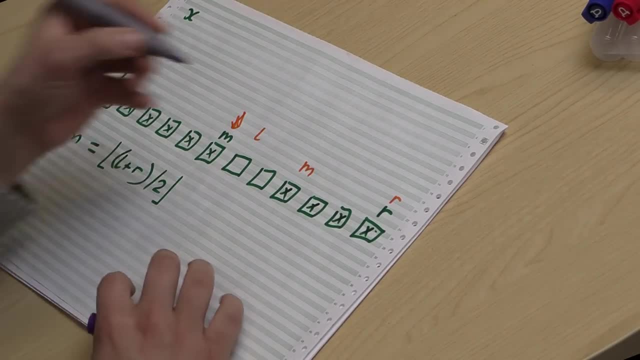 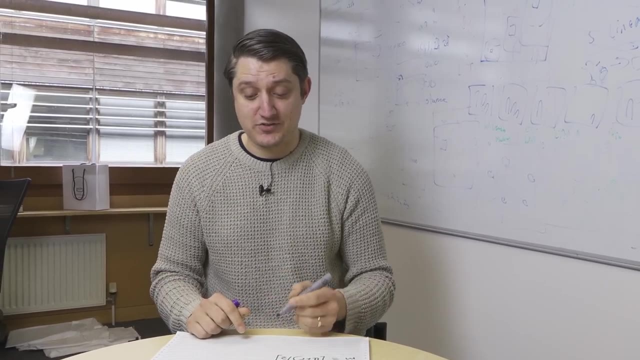 So we can now move new color Fancy Right. L stays there, R moves to here, All right, And we do L plus R divided by 2, which is actually going to mean that M is the same one here, All right. 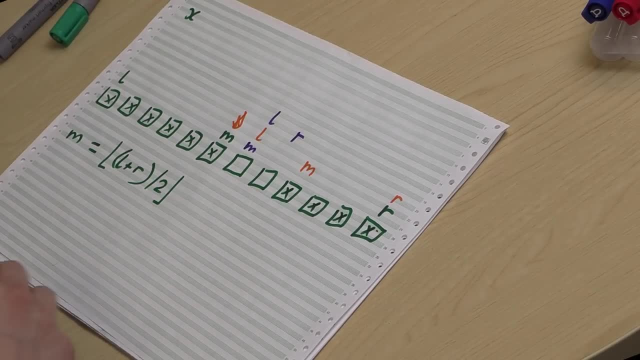 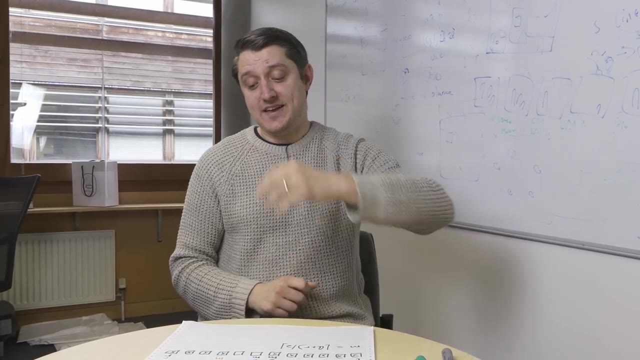 Like this. I should have done that above, And so we look in this one, and if M matches, then again we're finished. If not, we're going to have to go this way and so on, And what will happen eventually is you'll do this for however many items you have. 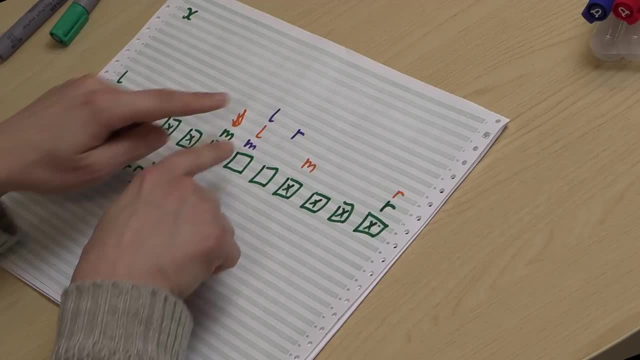 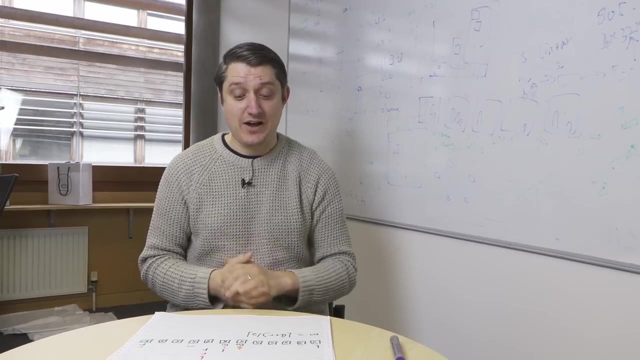 And eventually L and R will swap places because you'll move one of them this way or something like this. So if L is greater than R, or something like that, then you're finished. All right, And you haven't found it. Now, hopefully you do find it, but it depends on the problem. 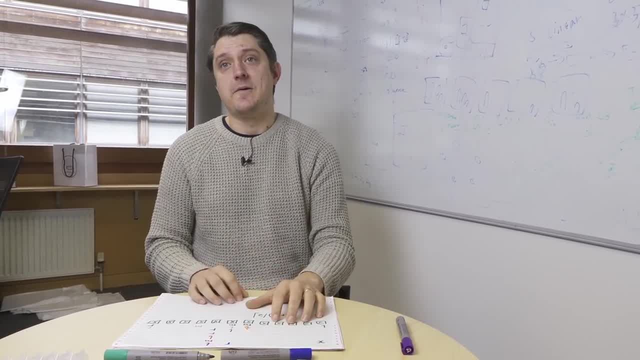 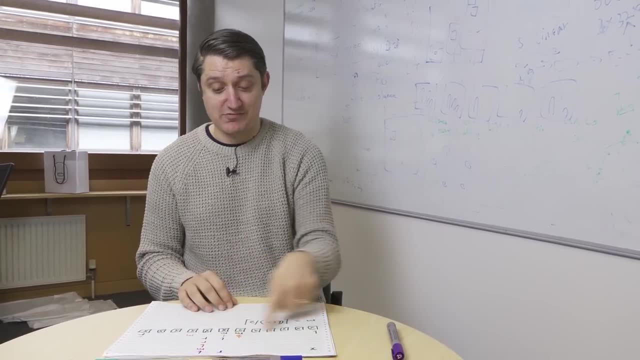 So hopefully you can see this is much, much faster than doing a linear search And actually it's not very difficult to implement because you've just got L, you've got the array, you've got R and M, Oh and X. 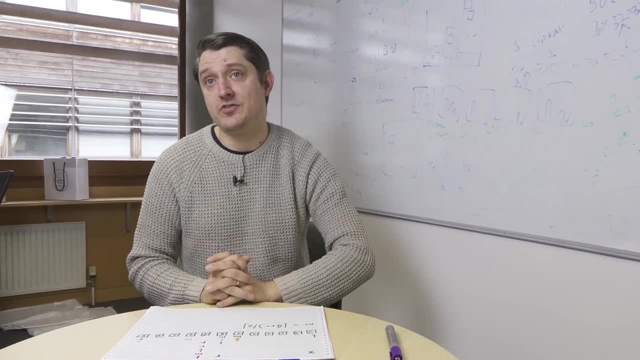 That's it. There's only a few variables, There's actually only a few lines of code, So let's write that up in Python and see how it goes. All right, So let's look at this. I've just whipped up this algorithm. 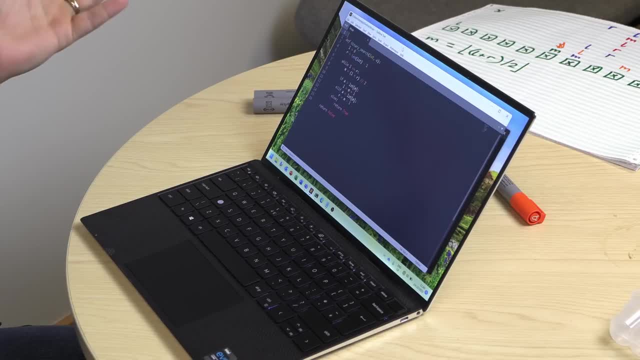 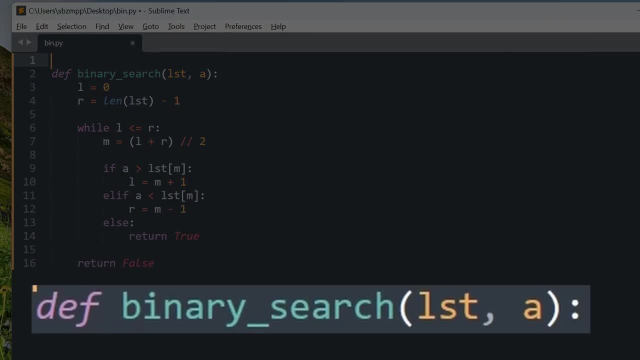 It's very, very straightforward. We have a function called binary search. That's a success, as far as I can tell. It takes a list, which I've called LST, and an A, which is our variable we're searching for. 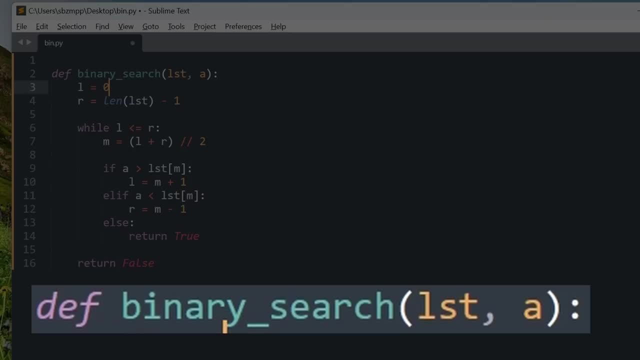 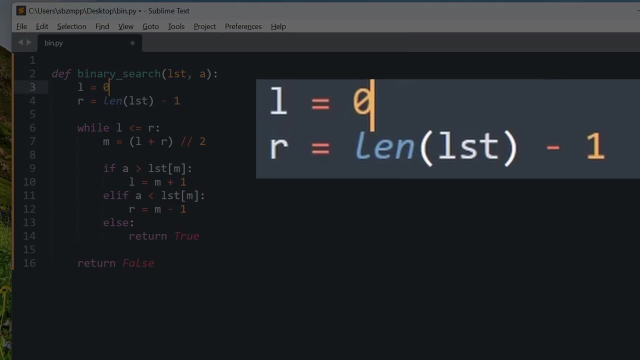 All right, So I've changed the name of the variable, just to confuse matters. We set our left to be zero, because in Python, zero is the first element of an array, And we set the right to be the length of the array minus one, which is the last element. 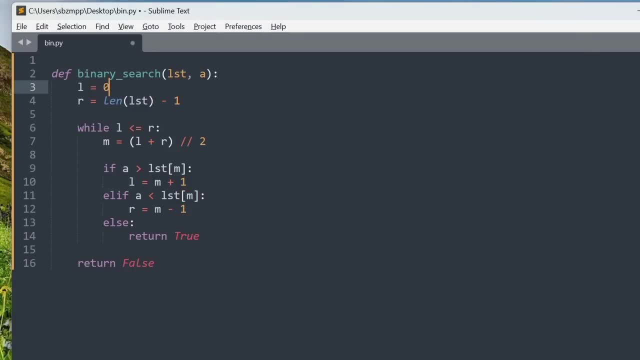 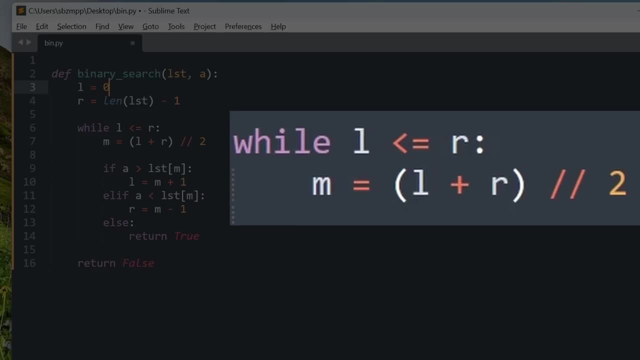 of the array, And then we have our loop. So we basically say, okay, while L is smaller than or equal to R, or less than or equal to R, we're going to repeat, We're going to calculate our new M, which is L plus R divided by two. 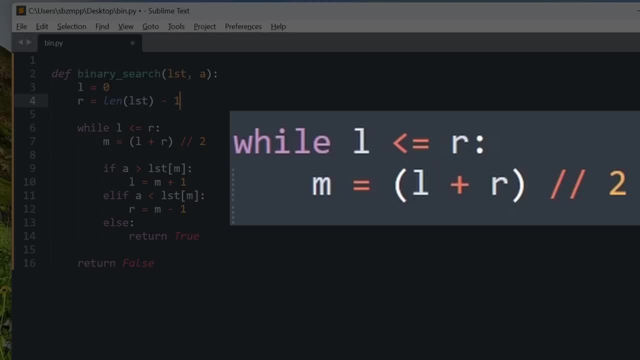 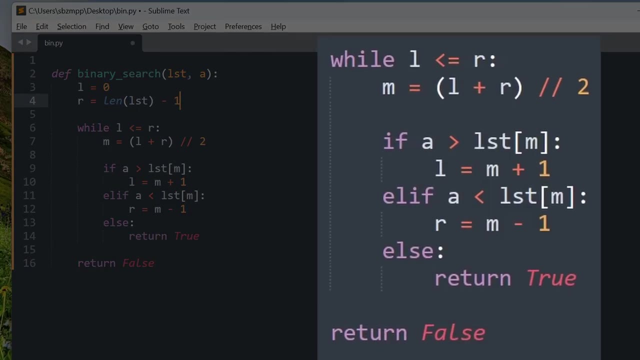 And here I've used the double slash to do an integer division. So basically it will automatically discard any fractional component. Then we say, okay, is a greater than the element M, in which case we set the left-hand side to be M plus one. 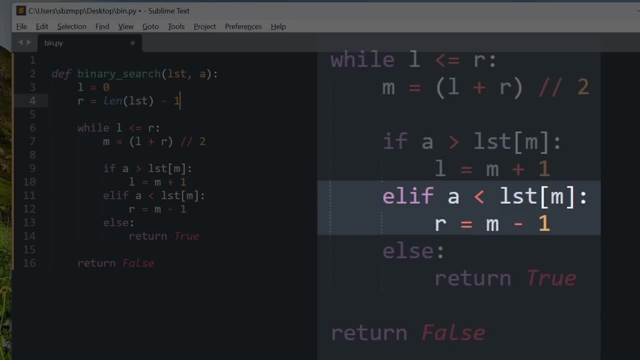 Or we say, okay, is a less than the element M, in which case we set the right-hand side to be M minus one. Or have we found the right number, in which case just return true, I'm not actually returning the number from the list. 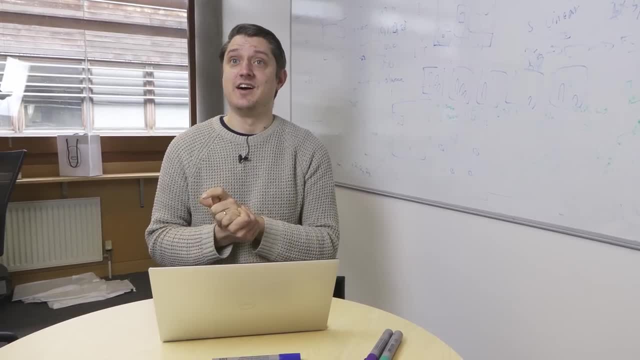 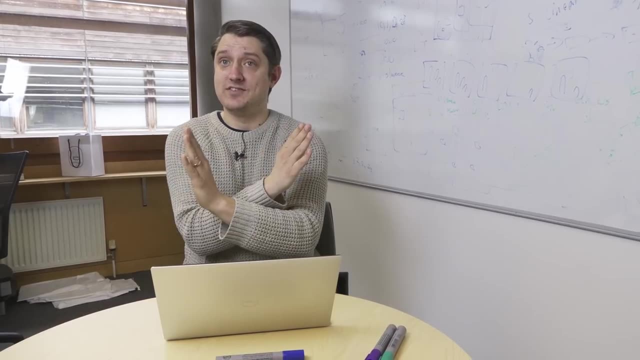 I'm just returning true or false, And that's the entire function. If we get to the end and L and R swap places, we just return false because the number wasn't in the array. So let's have a go, Let's see how much faster this is. 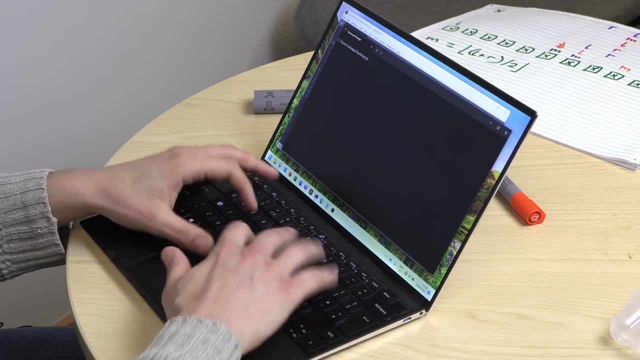 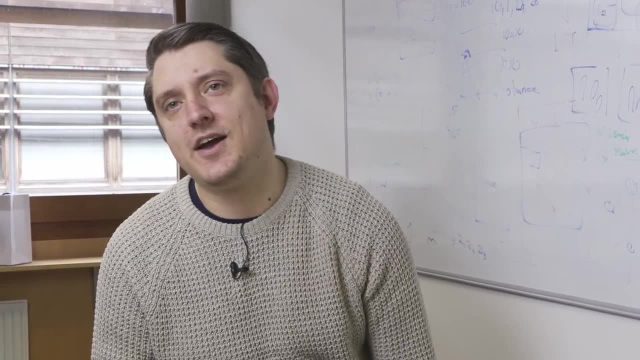 So I'm going to run Python here. So I'm going to run Python minus. i bin dot pi, which is my function. Well, how big is the array you're looking at then? Well, I'm looking at an array that is not so big that my computer dies. 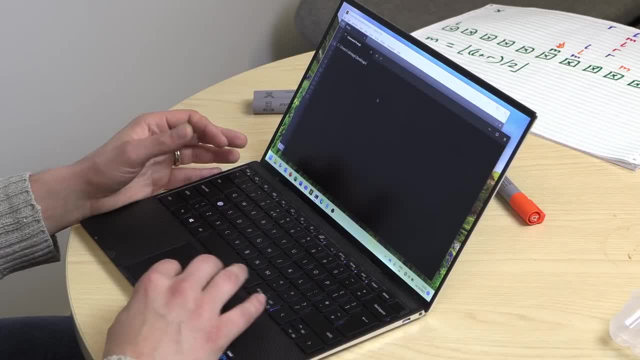 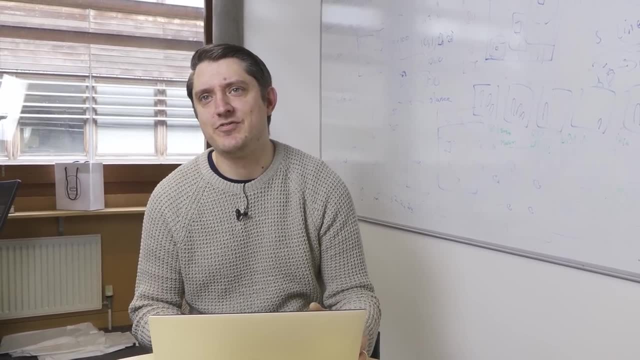 That was what I was really aiming for, So I've chosen the array: Two billion. No, sorry, no, I think 100 million. I think 100 million is right. Two billion might be pushing my laptop a bit far because there's a lot of overhead in the variables and things. 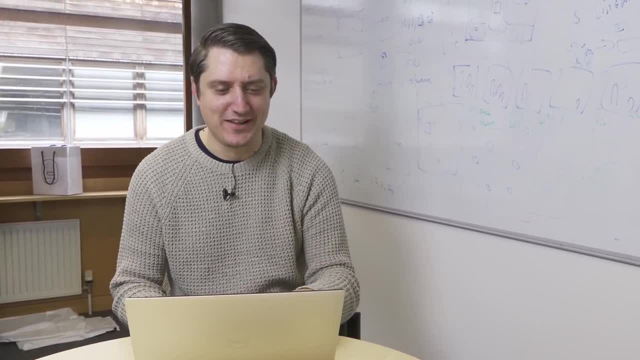 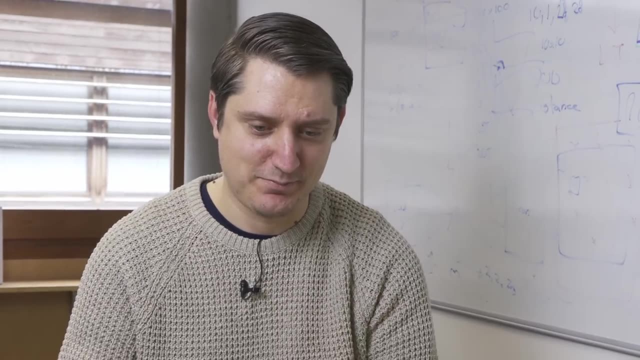 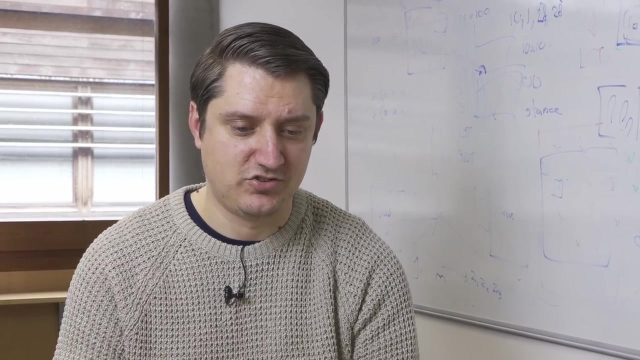 It just seems to be taking up quite a lot of RAM. I'm not overly. I'm not overly confident, Minus, i bin dot pi Right. So we run this and now it's loaded up my function So I can say binary search and it will show me. I've got a function there so I can look at it. 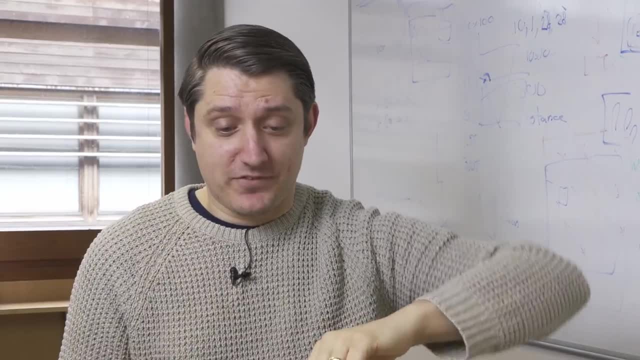 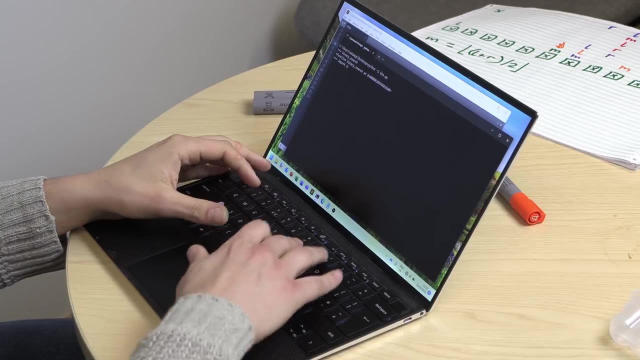 So now let's create a new list, and a big one. So what I'm going to do, I'm going to import numpy, because that's a good way of generating large lists of numbers. So import numpy as numpy. It's a new list. 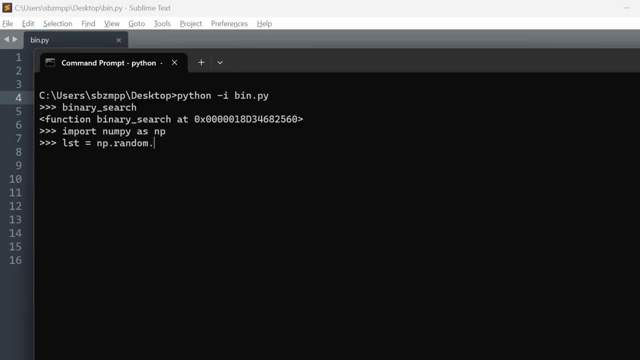 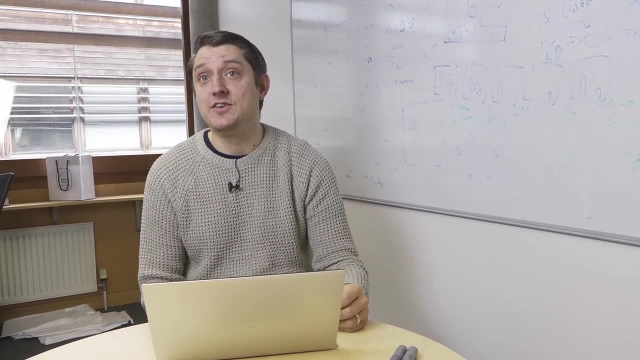 LST is equal to numpy dot, random dot, randint, So random integer, Let's not do decimals. And how big do we want? How many random ints do we want And what's the maximum value they can take? Well, let's make them two. 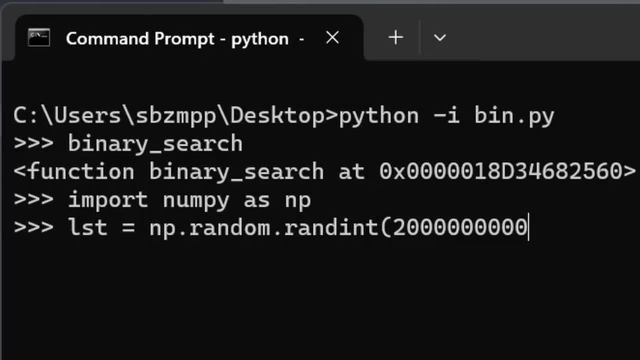 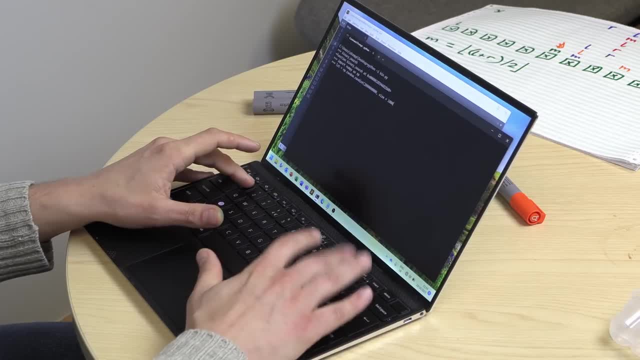 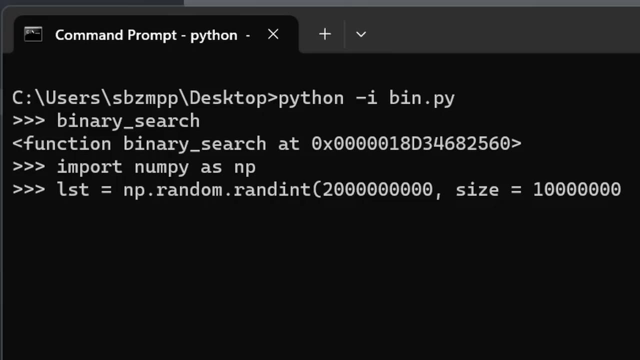 They're somewhere between zero and two billion in terms of the numbers, And let's say, size is equal to 10 million. So 10 million, So that'll be an array of 10 million items. that might be any number between zero and two billion. 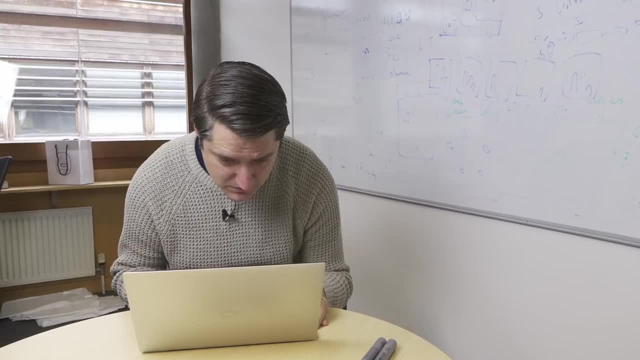 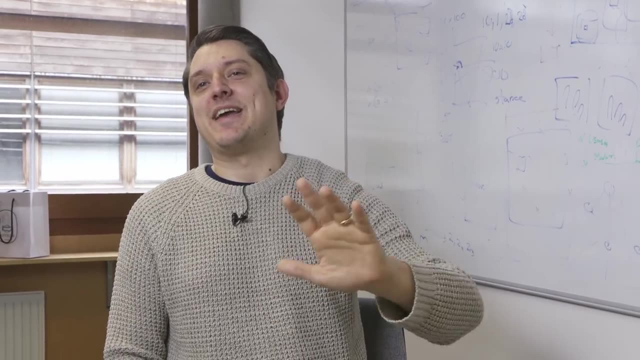 Two billion, yeah, So there'll be a little bit of repetition, but not a lot. And will that come out sorted? No, So let's push it out a bit. Let's make it 100 million. One more, But I'm going to copy this to a list: 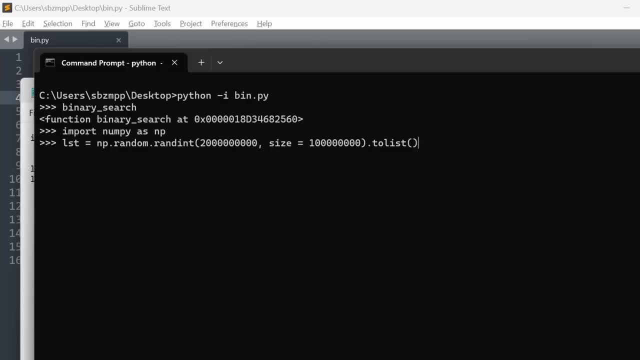 There may be a better way of doing this. I don't know what it is. This could just take a little minute. It won't take as long to do this as it will to sort it Where we might actually go and get a coffee first. 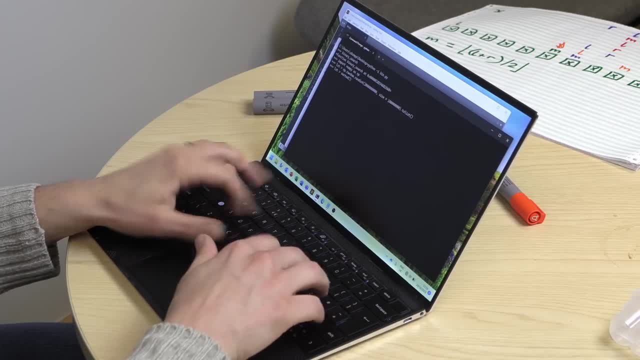 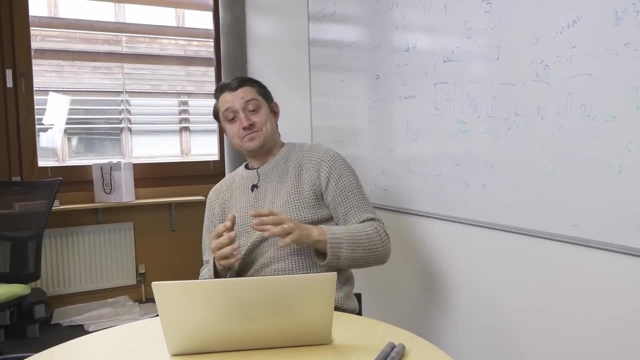 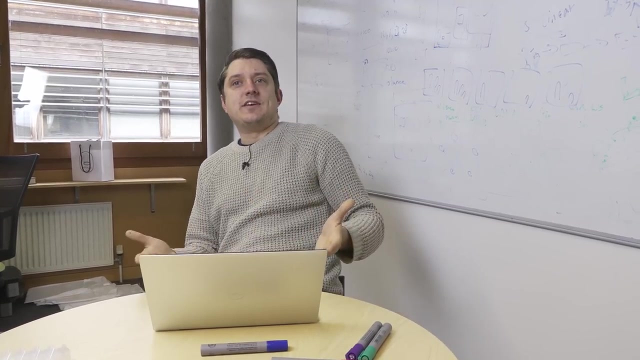 So now we're going to say lst is equal to sorted lst, And then we're going to have to just relax for a little bit because we've got some time to wait. Now, actually, this is quite an interesting point. Part of the interesting thing about binary search is that we're assuming the data is already sorted. 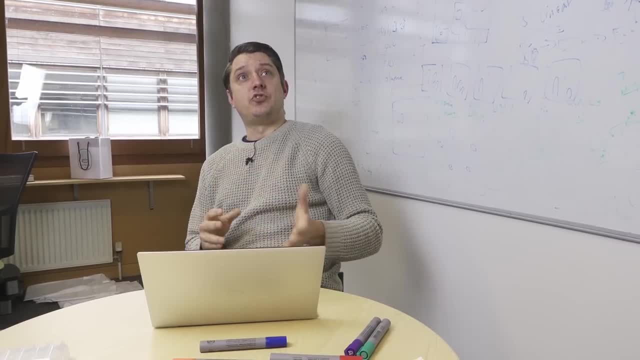 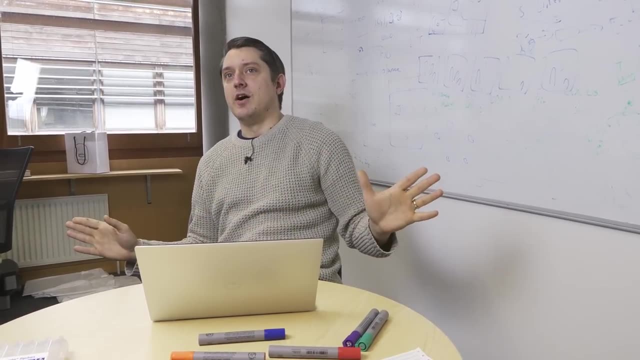 Now, sometimes that will not be the case, And sometimes sorting it is the real problem bit, And so actually, I think one of the really interesting things about things like binary search is you shouldn't just use it all the time. You use it when you're doing more lookups than you are sorting. 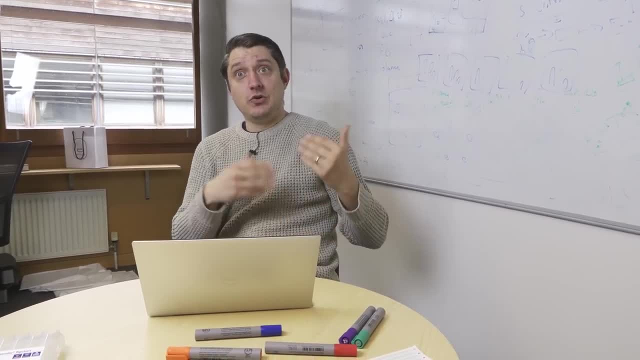 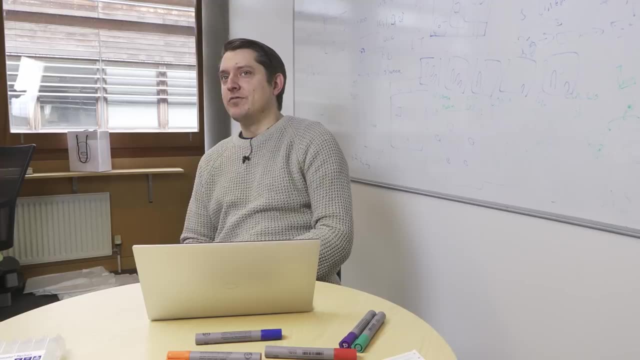 Maybe you sort your data at the beginning of the day for some reason, and then you just do lots and lots of lookups throughout the day. It makes a lot of sense to do something like this, Whereas if you only ever want to look up one value, you might as well just find it and not worry. 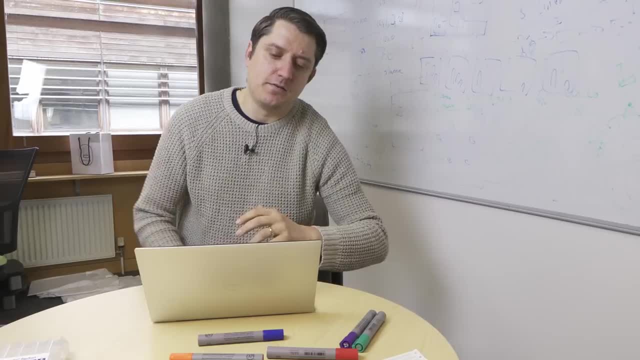 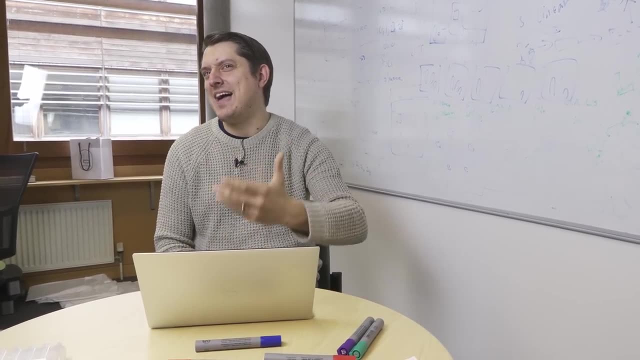 It's easy to mean. So I think actually, it's Rather than just learning all these algorithms. I think it's just interesting, if you're going to be a software developer, to think about when- Just to be aware of when- you should be using certain algorithms. 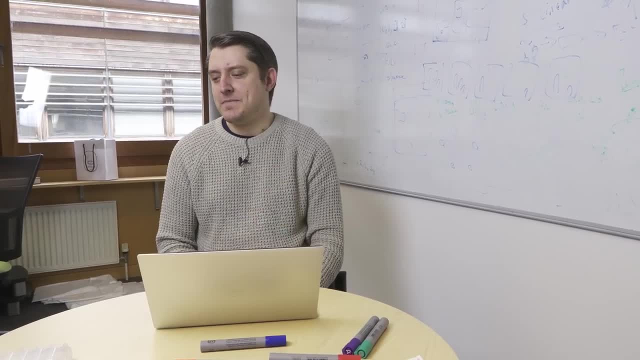 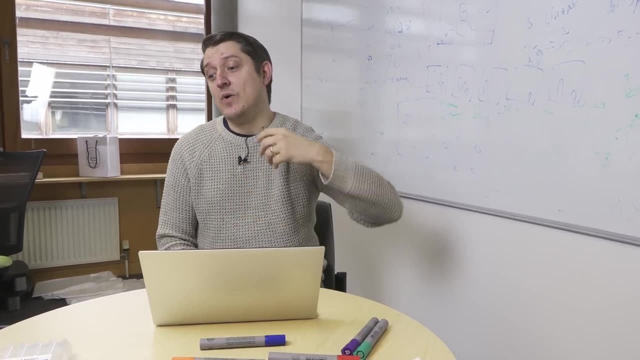 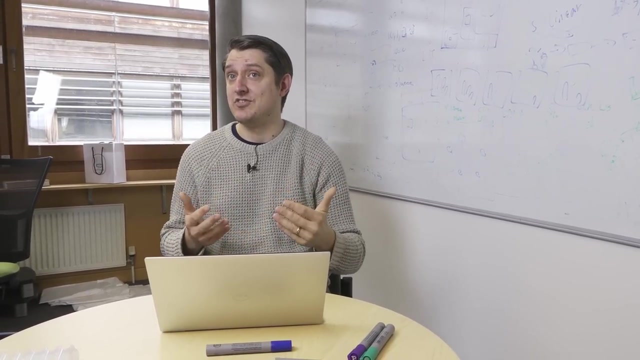 Whether it's appropriate. Yeah, Because you know there's a lot of people you know, can you program this kind of tree from scratch? Well, probably not. actually, I've forgotten how to do it. But what I can tell you is that you know, when I'm using a hash set or a list, I know roughly which algorithm would be the most appropriate in terms of efficiency for a specific task. 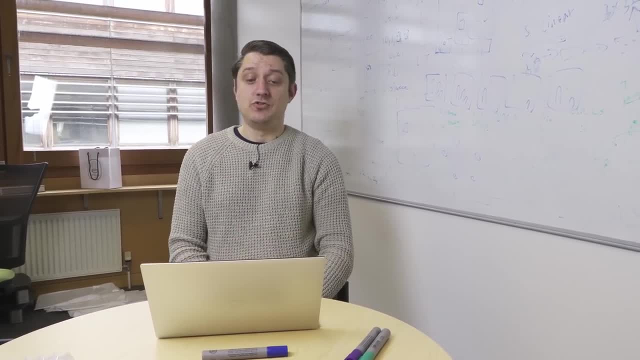 And I think that's a really helpful bit of knowledge to have, Because if you just use the default one, you'll often find it's quite slow. As we're about to find out, We're still sorting the list, by the way. 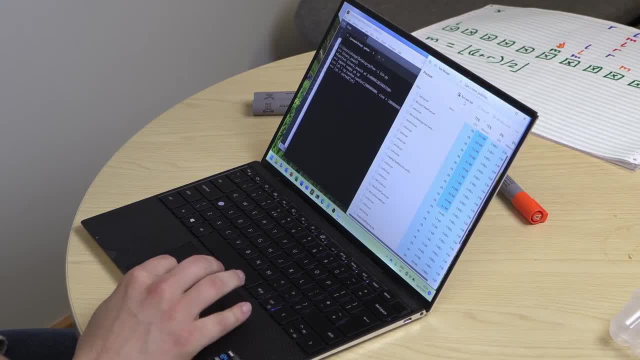 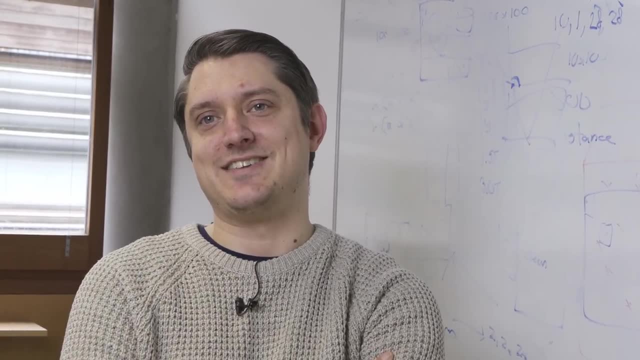 To be fair, this is a lot of numbers. How much RAM am I using? Oh, it could be worse. It's only 5 gig, But I couldn't. That would be. That would suggest I couldn't multiply my data set size by another 10.. 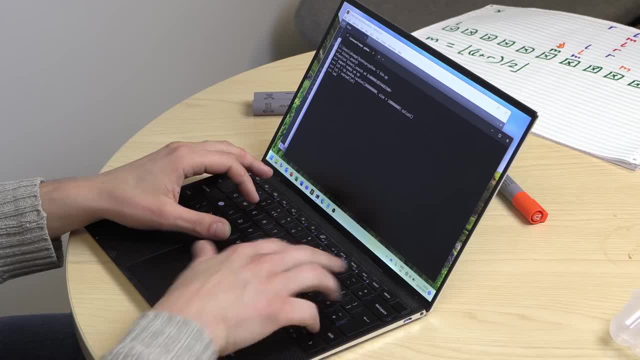 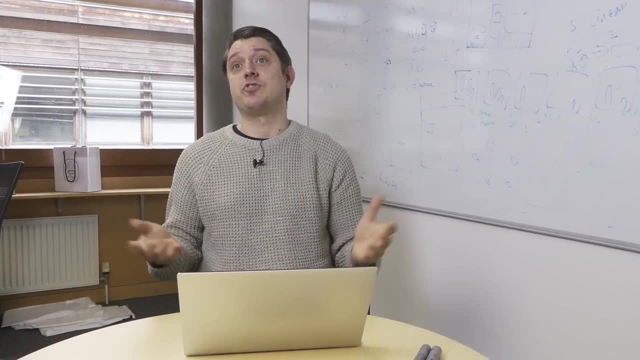 Although, Okay, sorted, That's good, Right. So if we type len of list, Right, It's 100 million. Right, I'm trying to. I think it's 100 million. We can, for example, select the millionth element to the millionth and tenth element. 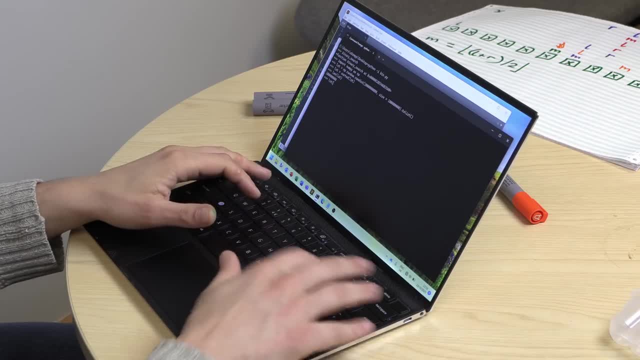 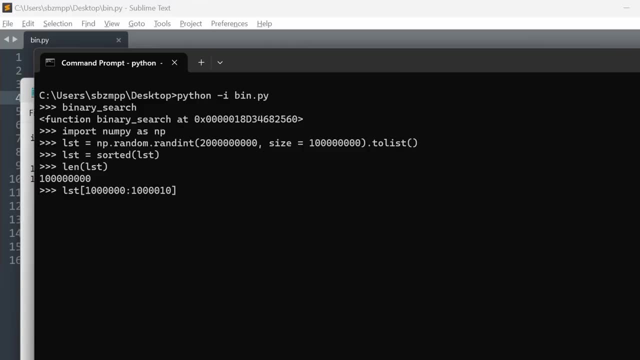 Right, So we could say list index from a million to there, Right? So that's All the numbers in this array from a million to a million, and ten position, And one of them is: Is 17 there? 17 is not there, would you believe. 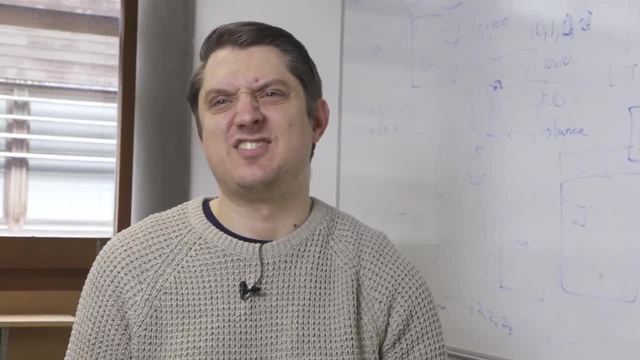 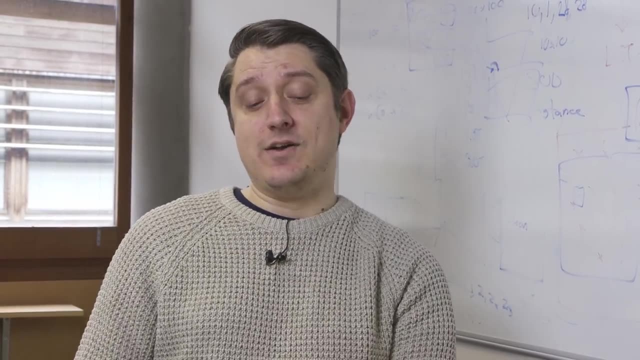 Now there will be a little bit of repetition in this array Because some of the random numbers will have turned out the same, But we're not going to worry about that today. So if we want to find out whether a number is in this array, all we need to do in Python. 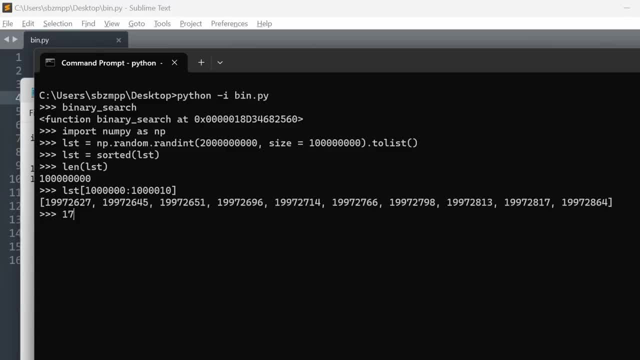 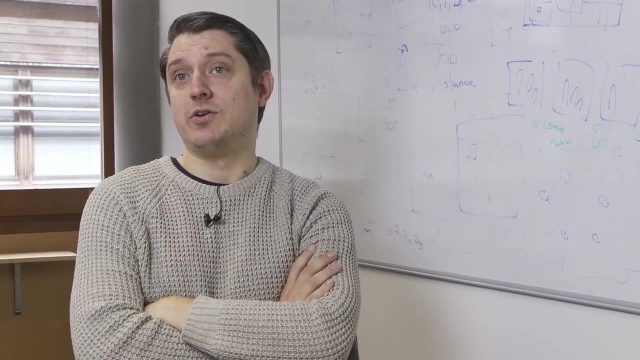 is use the in keyword Right. So I could say is 17 in LST And we sit here for a bit while it looks through every single number And it's not going to be in there False Right Now. why did that take so long? 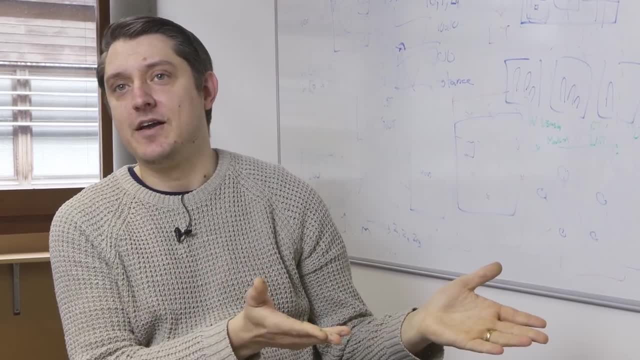 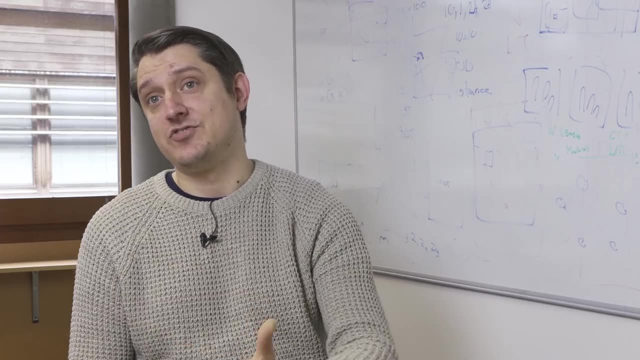 Right, Because 17 is going to appear right near the beginning. Right? Well, it's because Python doesn't know that this is a sorted list, Right? There's no reason for Python to know, So it has to use a generic algorithm like a linear search to solve this problem. 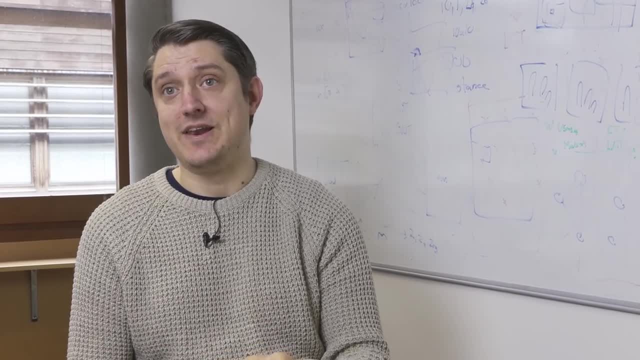 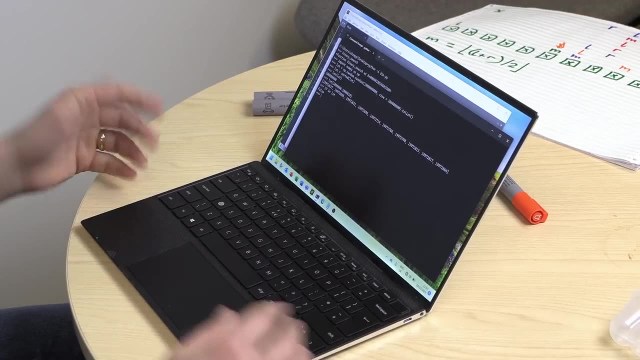 Right. So if 17 had been in, it would have returned very, very quickly Because it would have hit it right at the beginning. But it didn't, Right. So if I look at, If I search for this number, that I can already see is in the list. 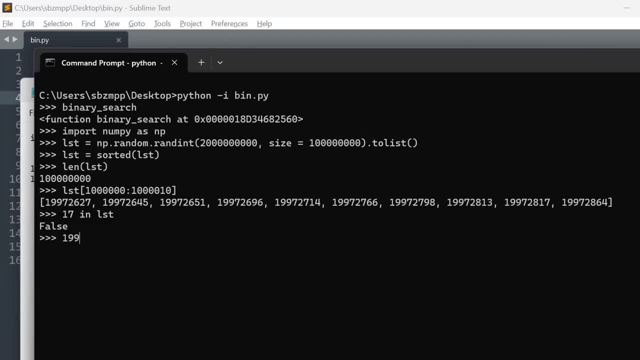 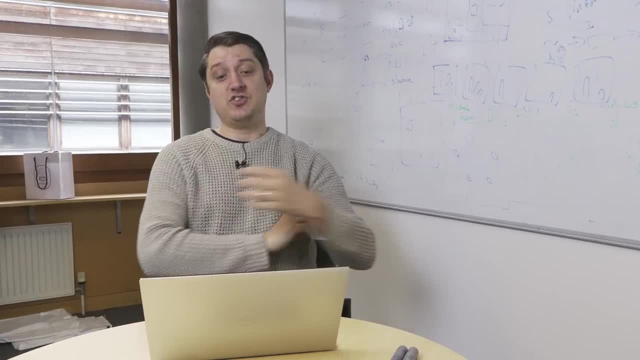 So if I say one, nine, nine, seven, two, six, two, seven in list, Right, It returns almost immediately Because it just goes a million in, finds it and stops Right. So sometimes you get lucky with this. 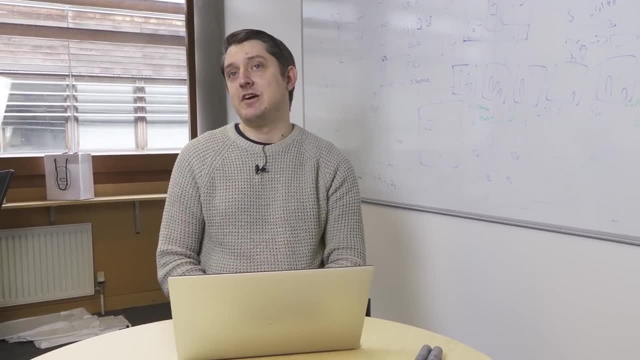 Sometimes you don't, But if you're just using the in keyword and your list is very, very long, you're actually just doing a really inefficient linear search, Right? So this is one of those times where you might think: okay, maybe this is a time when I need. 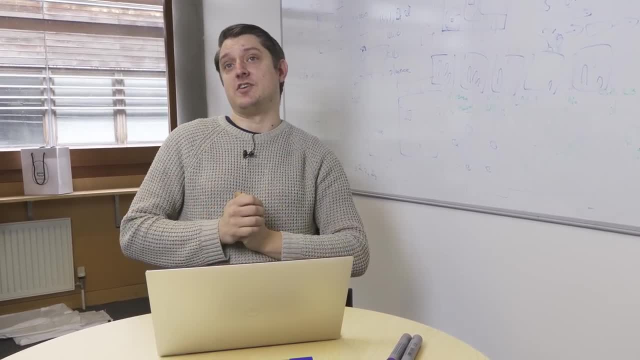 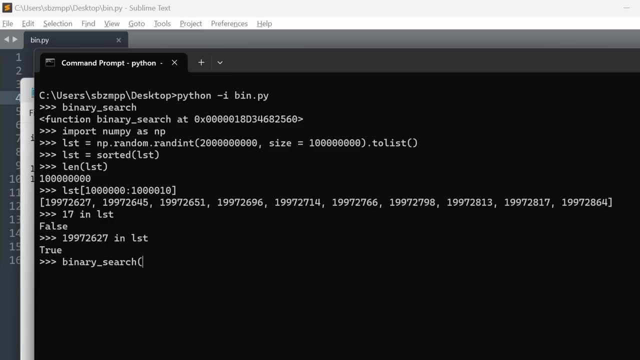 to find a slightly better algorithm to do this. So let's use our binary search and see if we can find some stuff in there. So, for example, binary search. So now you're going to use this. So now you're going to use that script that you've written. 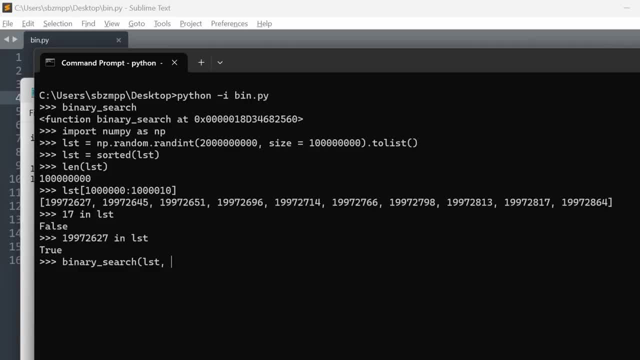 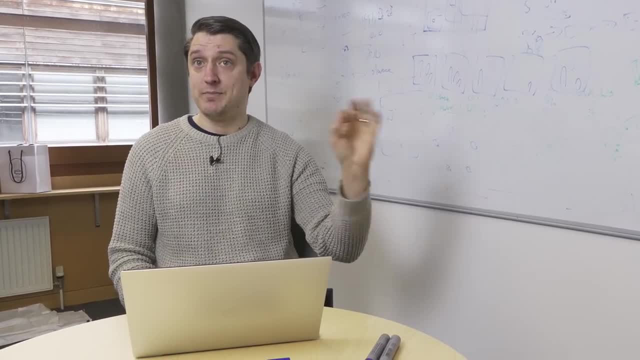 Yeah, So I'm using the function, I'm writing, I'm going to pass it the list, I'm going to pass it 17.. And it immediately returns false. Because it's just gone like this: doing a binary search, It's taken log to base two of 10 million right steps, which is 23.. 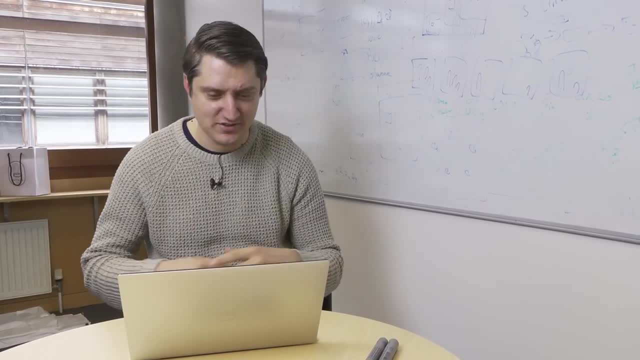 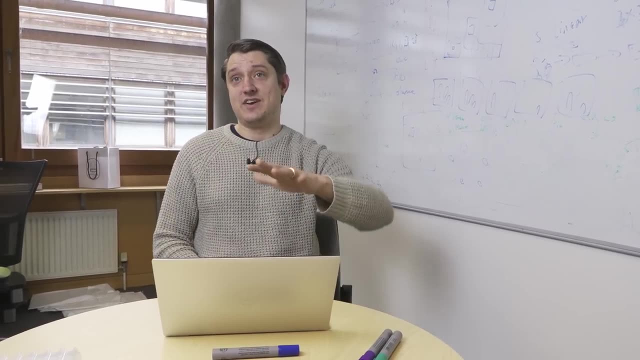 Right, So 23 steps and it got there. Yeah, Log to base: two of 10 million is roughly 20,, 22,, 23 steps. So it would have got there. So it would have got there. I mean, if you found the number on the first go, it might take fewer than that. 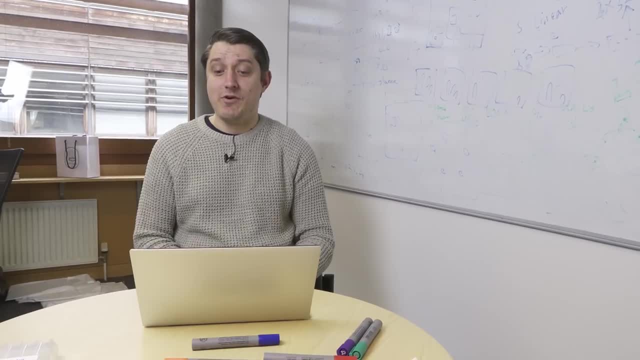 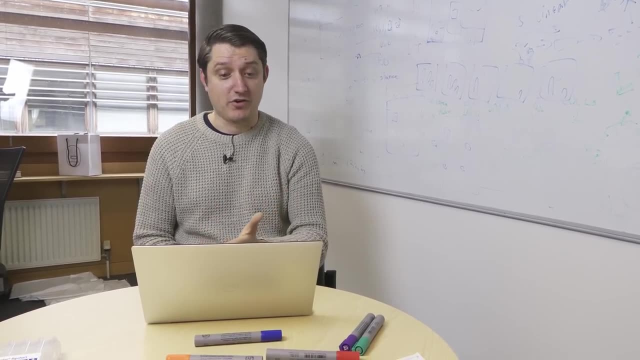 But in the worst case it's 23 steps, Whereas the worst case for finding 17 in this list of the linear search is 10 million steps. Sorry, 100 million steps, 10 times worse. So it's really bad. 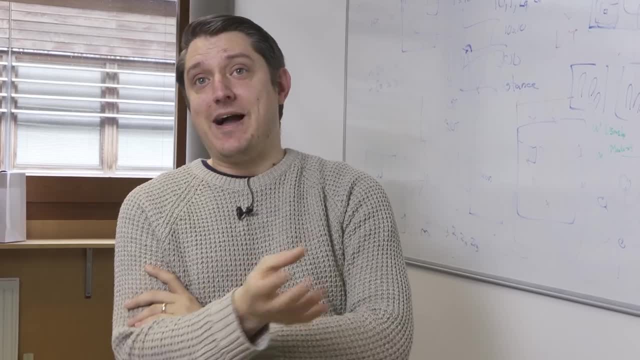 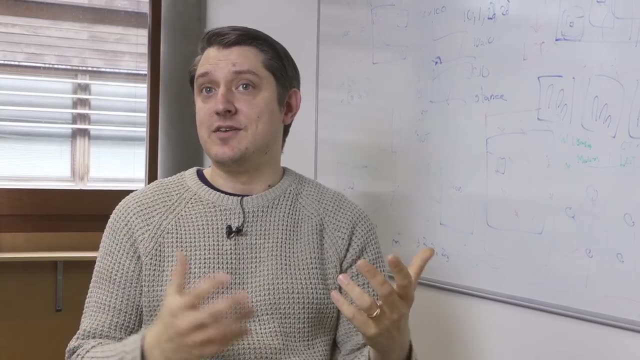 So this is a really, really powerful algorithm that gets used all the time, And extensions of this, where you have binary trees and you're searching through binary trees- is a similar principle, And the idea is that you've structured your data in such a way like we've sorted it here.